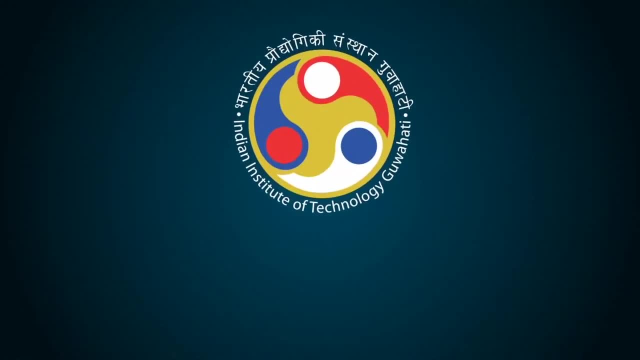 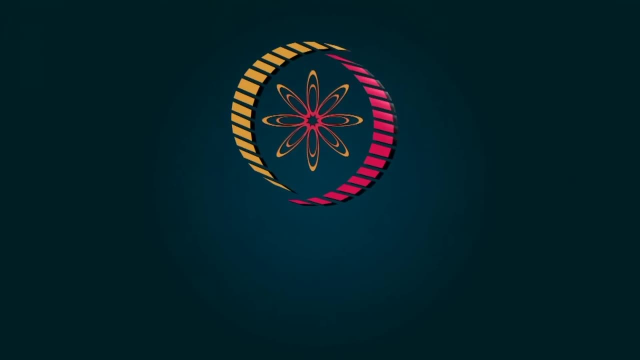 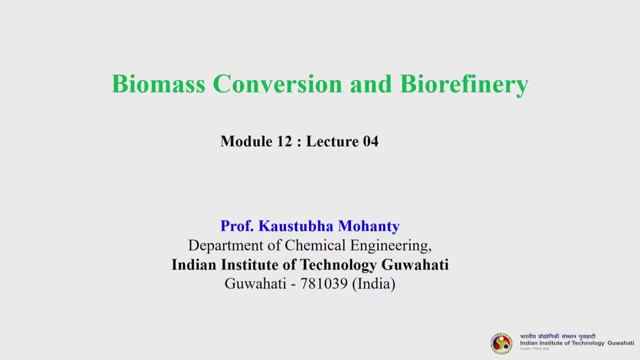 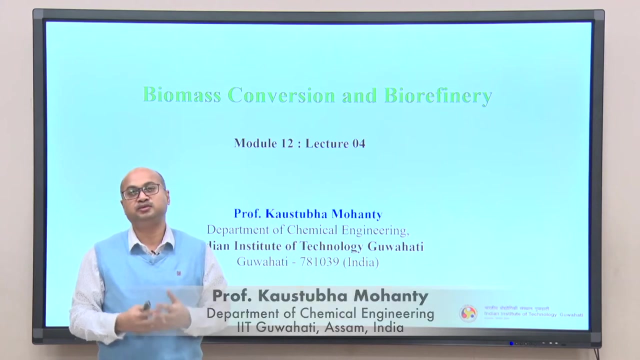 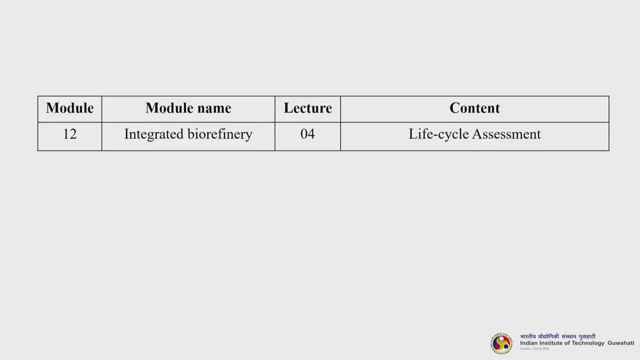 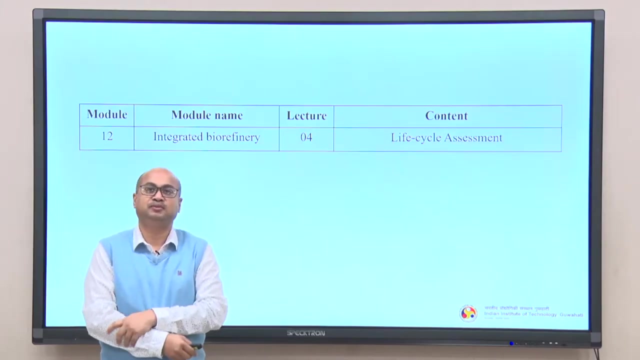 Good morning students. As you know, today is the last lecture of this module, as well as for this entire course, And under this particular lecture, under this module named integrated biorefinery, we are going to discuss about the life cycle assessment with a case study. As you know, that last class 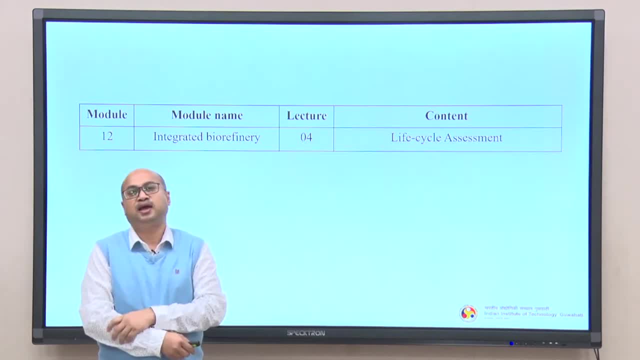 we have discussed about the techno-economical evaluation or assessment. Even in one of our previous modules we have discussed briefly about the TEA and LCA. But in this module we are going to discuss in detail about both TEA and LCA. TEA: we have discussed, LCA we 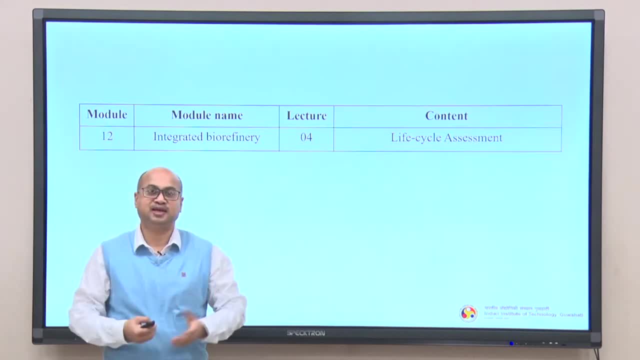 are going to discuss today. I will also take an example, or we can say a case study, that how LCA has been done or carried out for that particular biorefinery. So let us begin. Life cycle analysis, also known as life cycle assessment, is a primary 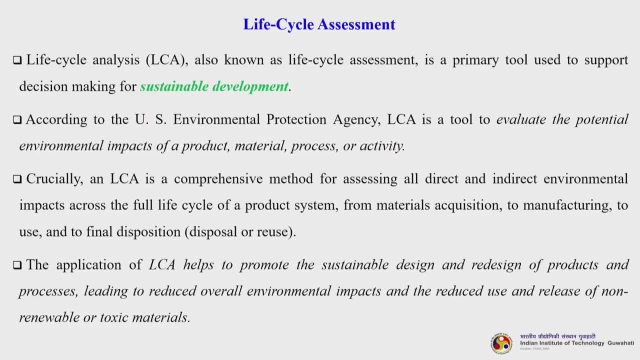 tool used to support the decision making for a sustainable development. According to the US Environmental Protection Agency, LCA is a tool to evaluate the potential environmental impacts of a product, material, process or activity. Crucially, an LCA is a comprehensive method for assessing all direct and indirect 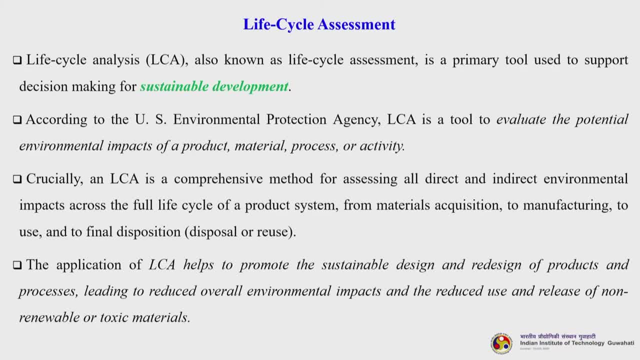 environmental impacts across the full life cycle of a product system, from materials acquisition to manufacturing, to use and to final disposition, or you can say disposal or even reuse. The application of LCA helps to promote the sustainable design and redesign of products And processes, leading to reduced overall environmental impacts and the reduced use and release of. 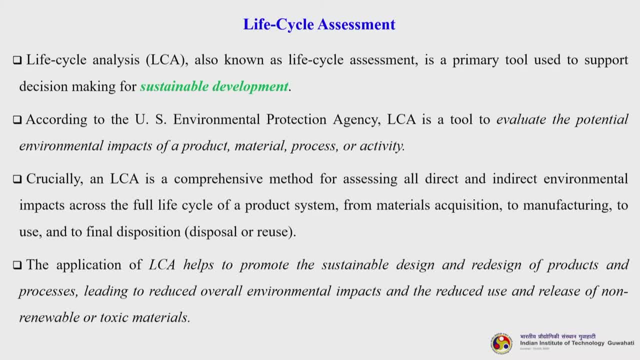 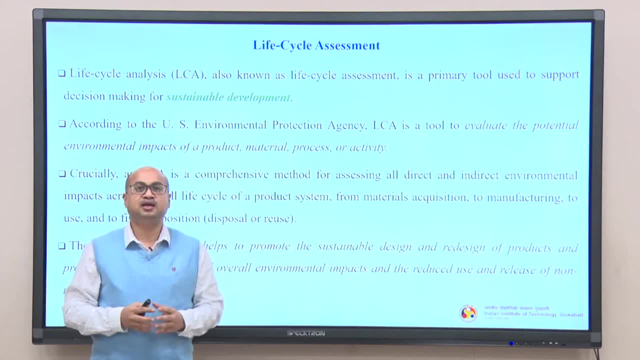 non-renewable or toxic materials. So, if you recall our earlier discussions, LCA is basically mostly relate itself to the environmental concerns: how a product which we are making in an industry- it can be any product- how it performs in its entire life cycle. 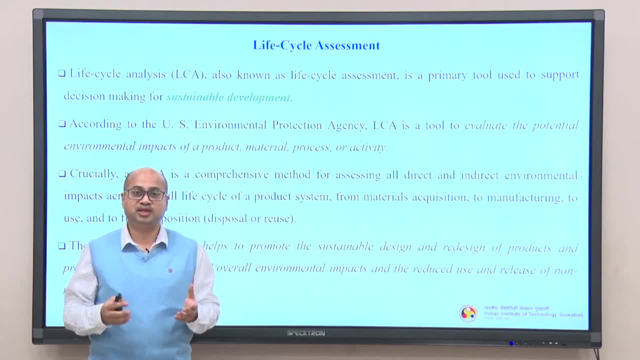 So that means we begin with the feedstock, then feedstock has been processed, converted product, it is purified, polished to a final product. then there are so many waste streams that comes out, okay, various types of waste. it can be solid, liquid, gas. how those wastes? 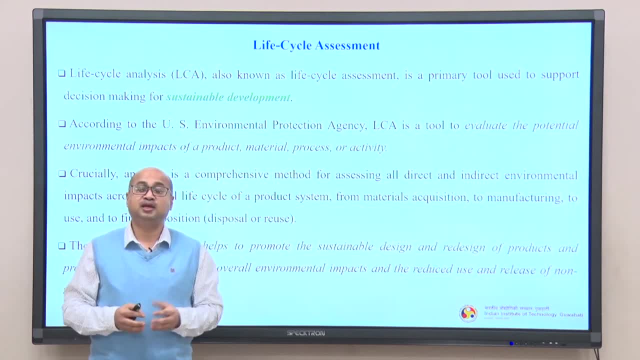 are being actually treated, how those wastes are being recycled and reused, and all these things are being covered in a life cycle assessment. So it tells us a comprehensive and overall view of how a product, once it is formed okay, is going to have a broad environmental effect during the life cycle. So this is a very 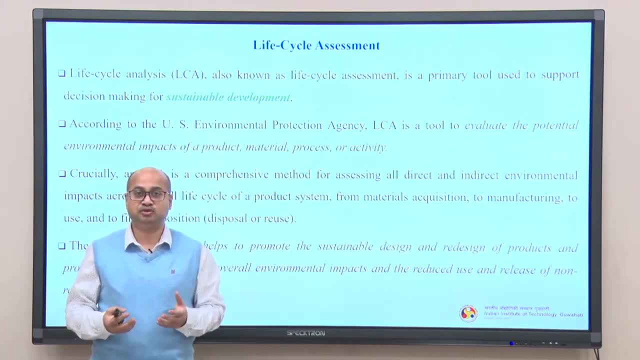 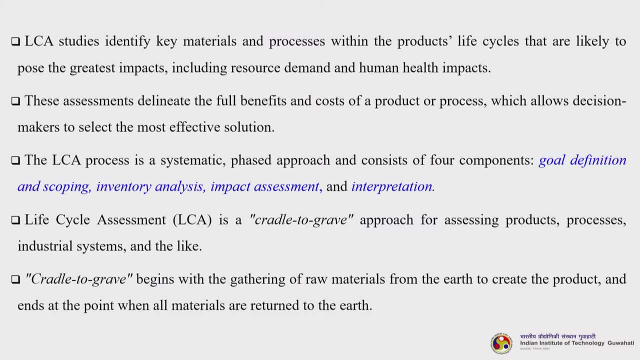 comprehensive and overall view of how a product, once it is formed okay, is going to have a broad environmental effect during the use as well as after the use also okay. So LCA studies identify key materials and processes within the product's life cycles. 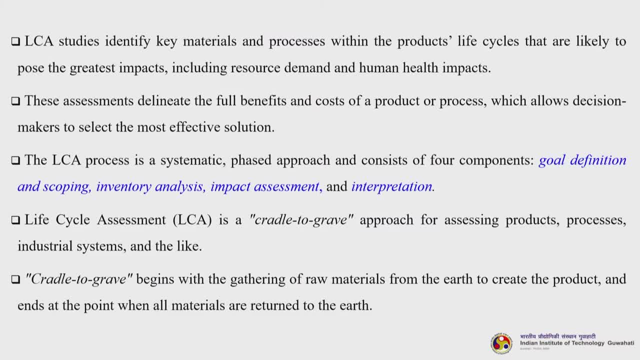 that are likely to pose the greatest impact, including that of the resource demand and human health impacts. Now these assessments delineate the full benefits and costs of a product or process, which allows decision makers to select the most effective solution. The LCA process is a systematic 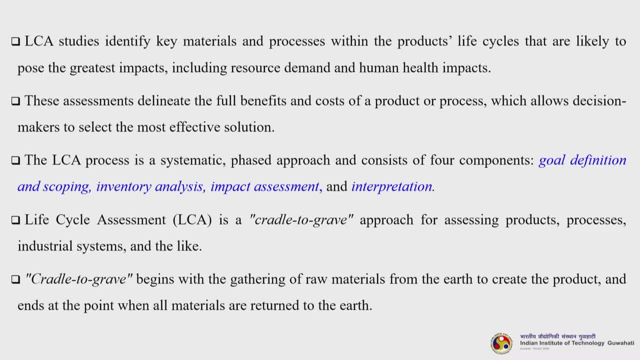 phased approach of four components. what are those four components? the first and foremost one is the goal definition and scoping. what is the scope, okay, and how you define it basically. second is that inventory analysis. third is impact assessment and last one is the interpretation. now, all these things. 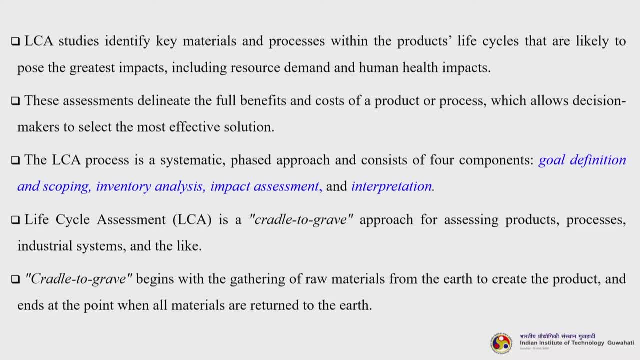 we will discuss in subsequent. this one slides today itself, okay, and when I take a case study so it will be more clear to you. so lifecycle assessment is a cradle to grave approach for assessing products, processes, industrial systems and the like. Cradle to grave begins with the gathering of raw materials from the earth to create. 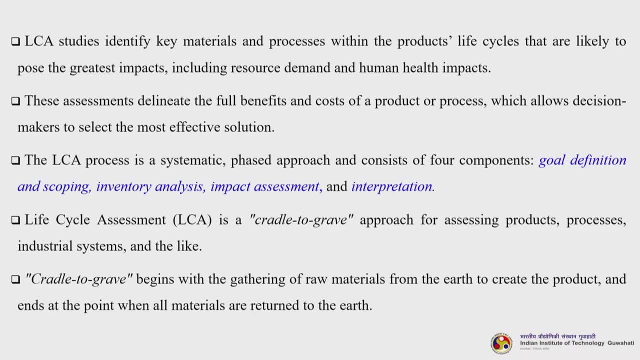 the product and ends at the point when all materials are returned to the earth. so this is a more holistic approach. when we talk about cradle to grave, okay, it starts from a point where it ends in the same point, basically okay, so it is a cycle. 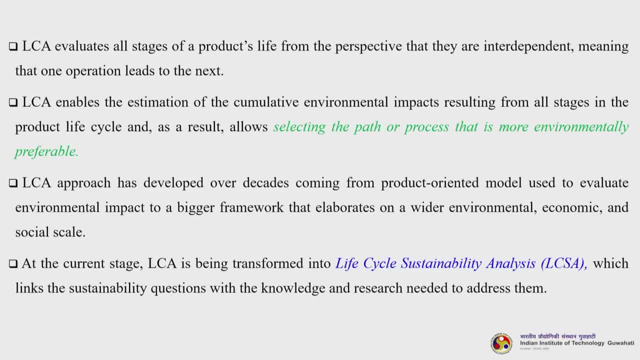 So LCA evaluates all stages of a product life from the perspective that they are interdependent, meaning that one operation leads to another, the next LCA enables the estimation of the cumulative environmental impacts resulting from all stages in the product life cycle and, as a result, allows selecting the path or process that 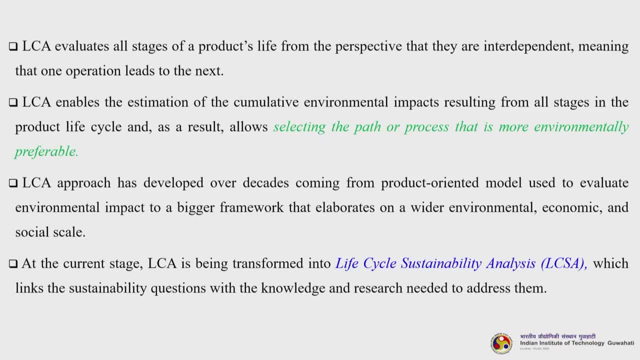 is more environmentally preferable. LCA approach has developed over decades, coming from product oriented model used to evaluate environmental impact to a bigger framework that elaborates on a wider environmental, economic as well as social scale. Social is also very important. okay, now, at the current stage, LCA is being transformed into life cycle sustainability. 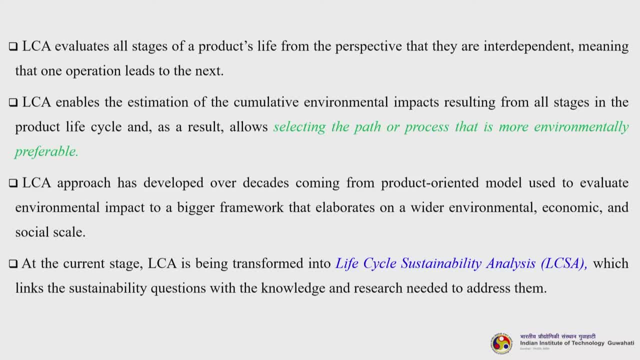 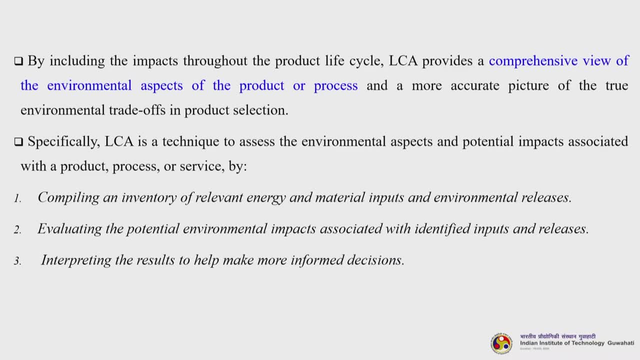 analysis, which people call it as a LCSA, which links the sustainability questions with the knowledge and research needed to address them Now. by including the impacts throughout the product life cycle, LCA provides the comprehensive view of the environmental aspects of the product or process and a more accurate picture of. 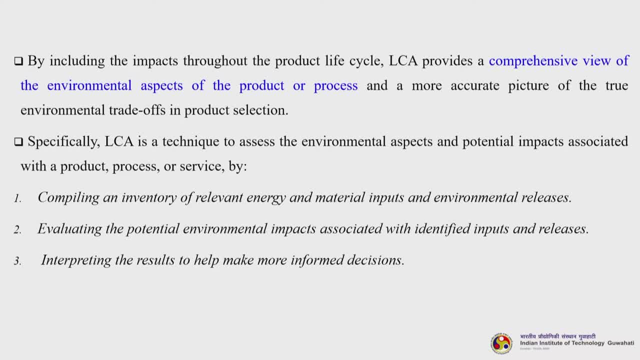 the true environmental trade-offs in product selection. Specifically, LCA is a technique to assess the environmental impact. First, evaluating the environmental aspects and potential impacts associated with a product, process or service by compiling an inventory of relevant energy and materials inputs, as well as the environmental releases. Second, evaluating the potential environmental impacts. 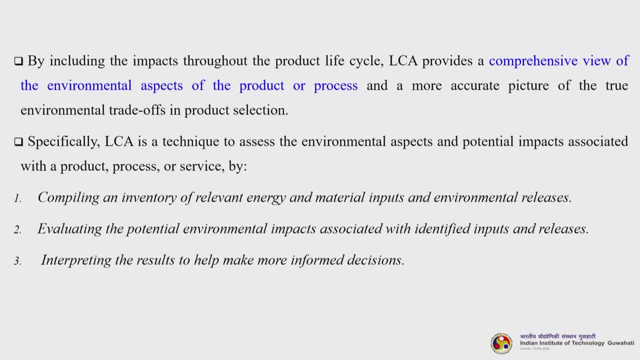 associated with identified inputs and releases. Third is interpreting the results to help make more informed decisions. So all these points are going to help us when we carry out this LCA or LCSA. okay, So you can have a look at this figure one. 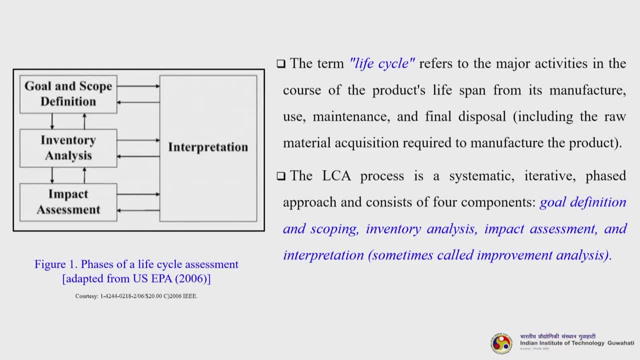 So this describes the phases of a life cycle assessment. okay, it was adapted from US EPA. okay. So goals, scope and definition, inventory analysis, impact assessment and interpretation. Now, all these things are interrelated with each other. so that means once the goal and 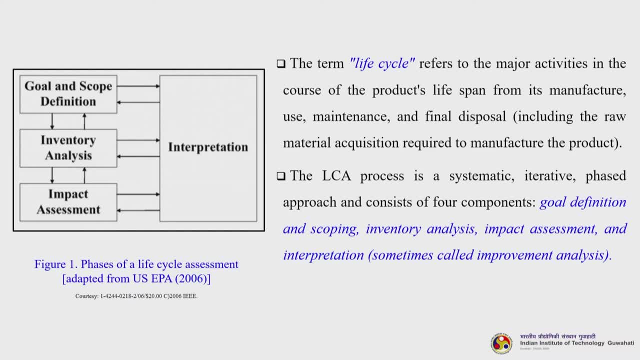 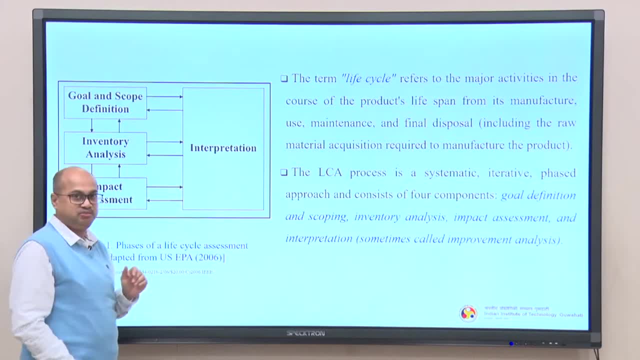 scope definition- okay, can be interpreted, and then that same can be used by inventory analysis. Inventory analysis data can be interpreted, okay, that same can be used to do the impact assessment. That means basically the meaning is that all these three parameters- the first two parameters- 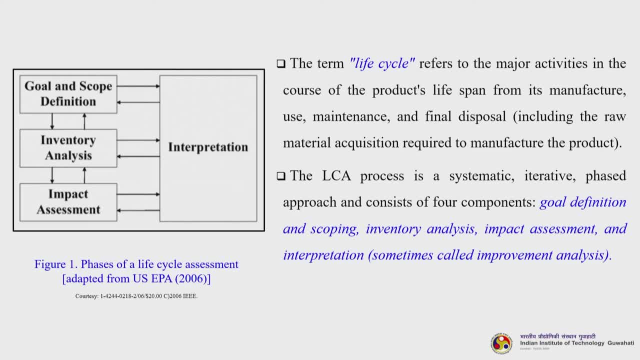 the second thing is the日本as and the last thing is the kettles. Understand therefore the basic parameters. they are interdependent in each other. So the term life cycle refers to the major activities in the course of products: lifespan from its manufacture, use, maintenance and final disposal. 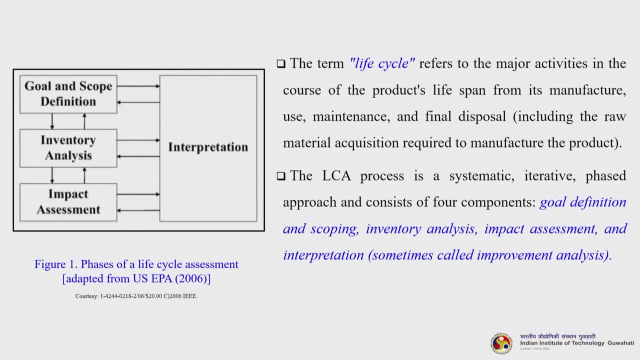 Now that final disposal. again, as I told you earlier also that, including the raw material acquisition required to manufacture the product, The LCA process is a systematic, iterative, phased approach and consists of four components: goal definition and scoping, inventory analysis, impact assessment and interpretation. Now, sometimes, if this also calls improvement analysis, ok, 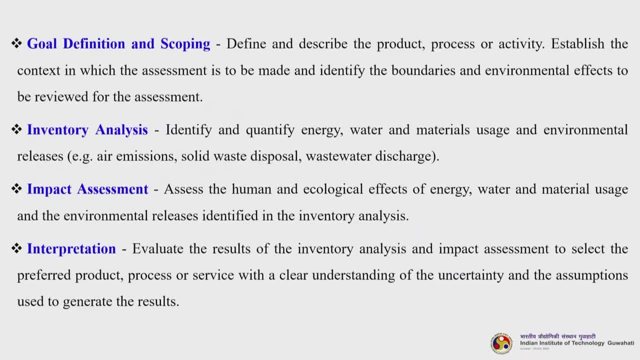 So let us understand what are these four parameters? so, goal definition and scoping: Now define and describe the product, process or activity, establish the context in which the assessment is to be made and identify the boundaries and environmental effects to be reviewed for the assessment. Then next is the inventory analysis. now, here you identify and quantify the energy, water. 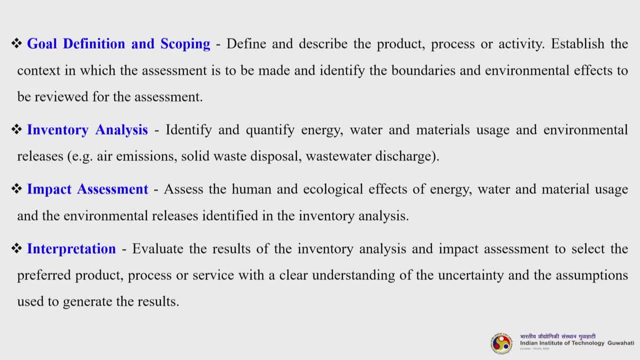 and materials uses and environmental releases, as, for example, air emissions, solid waste disposal, waste water discharge, all these things. Then, third, is the impact assessment. now assess the human and ecological effects of energy, water and material uses and the environmental releases identified in the inventory analysis. and the last one is interpretation. 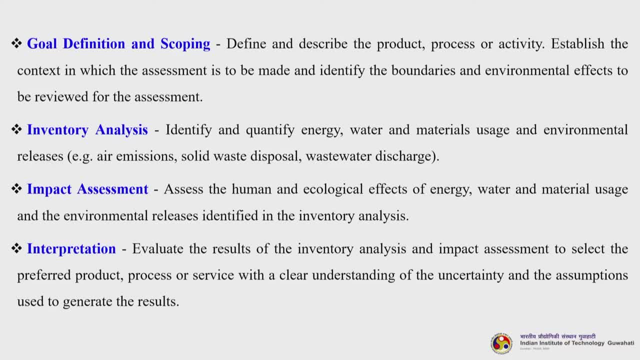 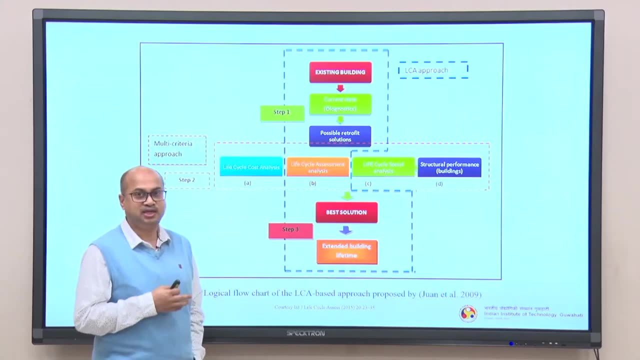 Now, here you evaluate the results of the inventory analysis and impact assessment to select the preferred product, process or service, with a clear understanding of the uncertainty and the assumptions used to generate the results. Now please have a close look at the figure 2, which tells us about. this is the logical. 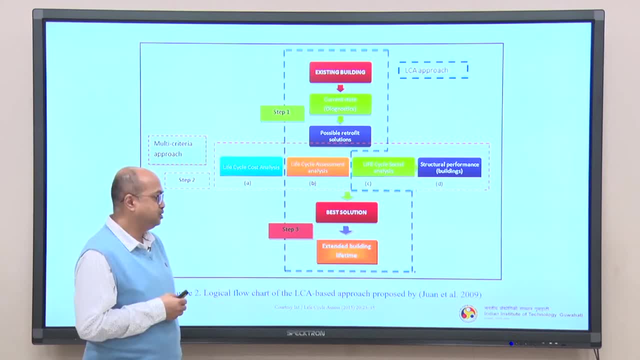 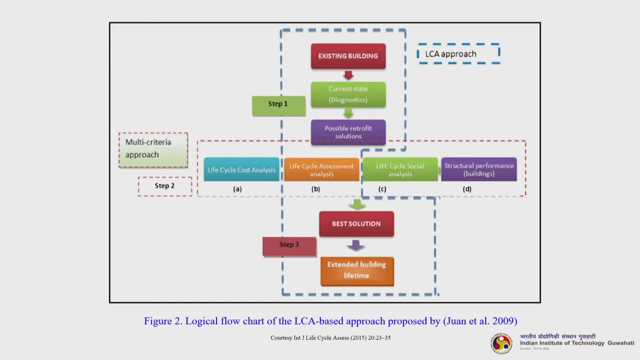 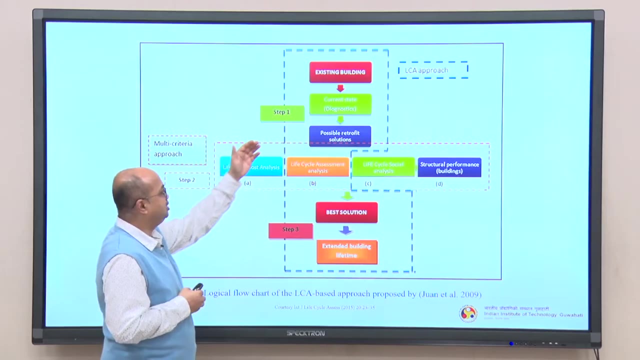 flowchart of the LCA based approach- ok, proposed right by Zouan et al. and this life cycle. this is international journal of life cycle, SSS, So this is being taken from one particular paper which is given in the below. So what it says basically. so it is telling us about the three different steps, ok. 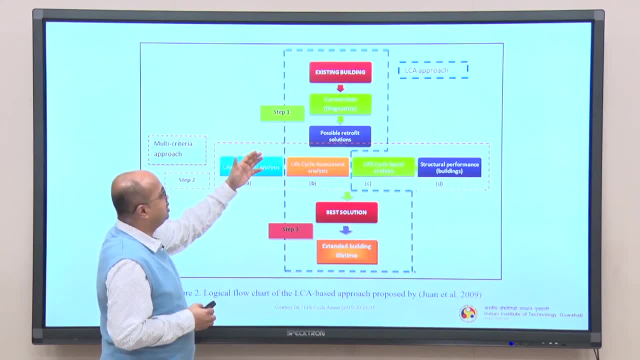 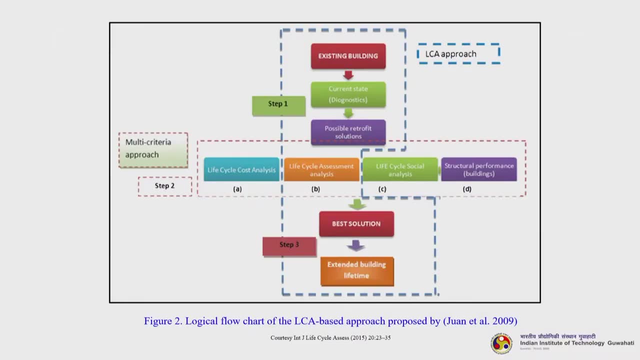 So step one, which basically talks about the existing building, current state, that is the diagnostic approach, then possible retrofit solutions. Now in the step two, it is a multi-criteria approach. here the life cycle cost analysis is there, life cycle assessment analysis, life cycle social analysis and structural performance. 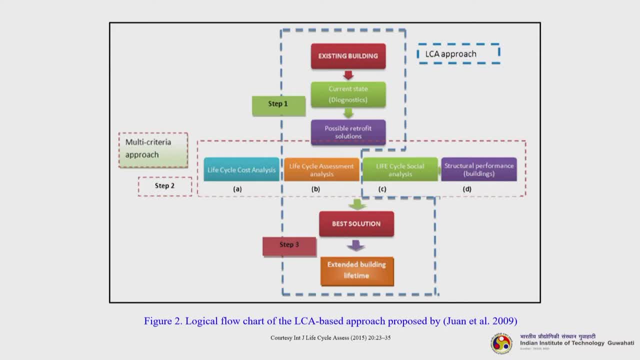 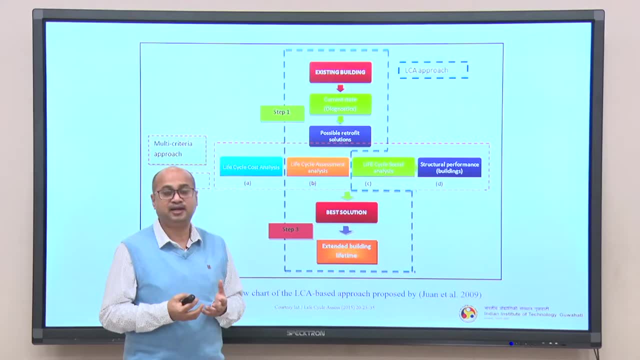 again buildings. ok. Now the third one is which out of all these, when we collect data and analyze them, analyze the impact, analyze how they are going to create problems for environmental effects and all these things, Then we can think about the different types of solutions. 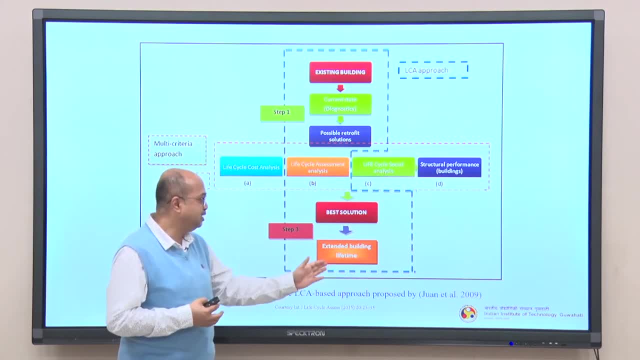 Now, out of that, you have to go for a best solution. then extended building lifetime and, as you know that all these- again I am telling you, they are all interdependent on each other. one particular parameters data will have enormous effect on the subsequent conversion processes, subsequent wastewater treatment processes, subsequent energy requirement and all these. 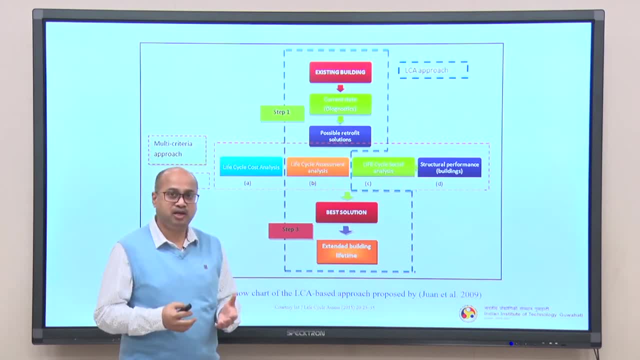 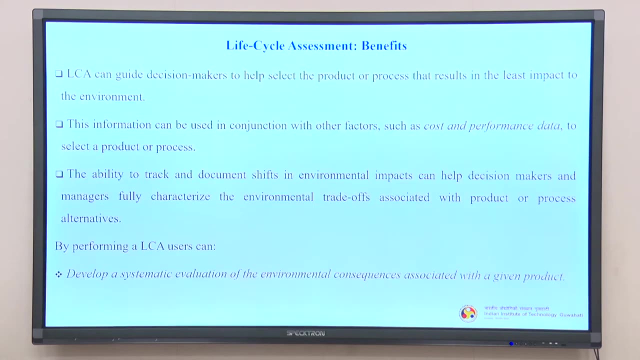 things. and from the upstream side also, when you talk about procuring raw material processes, Then making into a particular shape, size, density, so that it can be stored properly and can be used for further conversion. so all they are related to each other. So let us understand the benefits of the life cycle assessment. now LCA can guide decision. 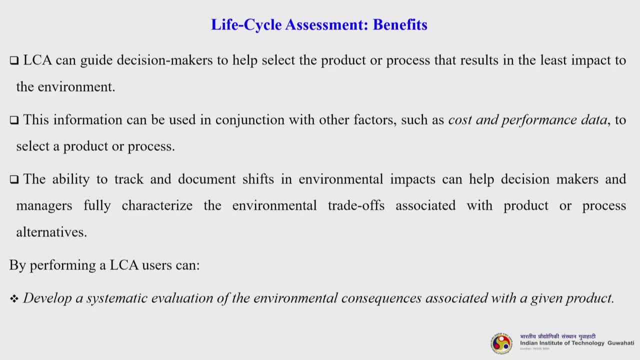 makers to help select the product or process that results in the least impact to the environment. Now this information can be used in conjunction with other factors, such as cost and performance data, to select a product or process. Thank you. Now again, I am telling you. there are two important things, if you remember, in our TA discussion. 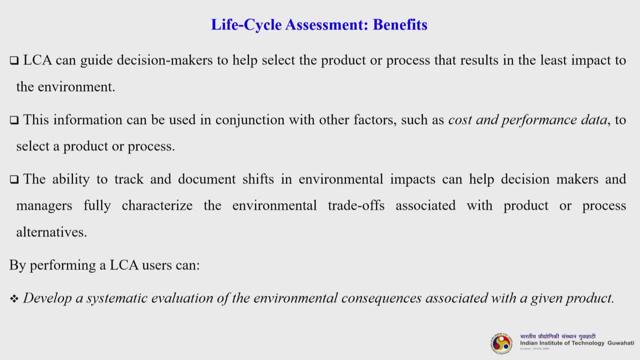 I was telling you. it is very important to understand that if somebody goes for development of a process, a technology, then find out whether it is technically valuable or not. that is a technical part. then the second is that whether it is techno economically valuable or not- okay, or sustainable or not. and third is the life cycle assessment. 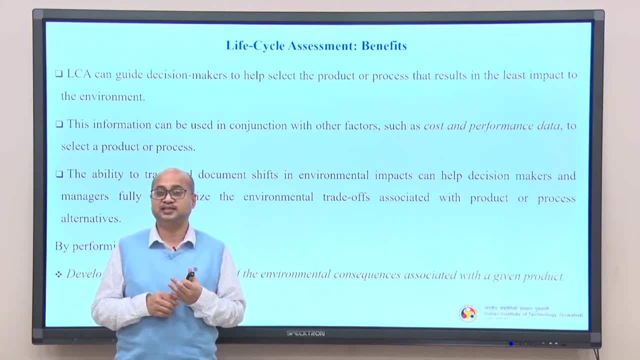 So all these three things you have to do, first is technical challenge, second is the techno, economical challenge- Okay, Let us say the cost of the product and the process- and third is the life cycle, which takes into account also a part of the processes which I have discussed earlier. 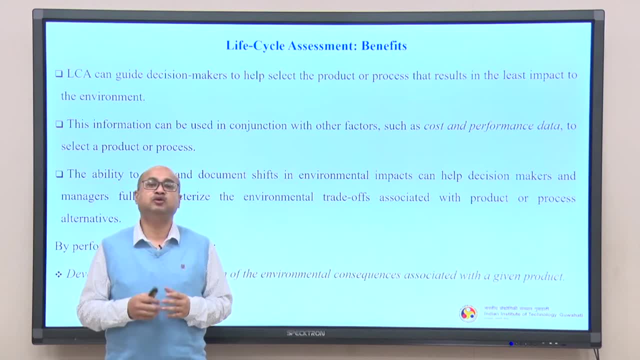 So all these things will be taken into consideration when somebody goes for building up a new biorefinery or a refinery or any process industries or any industry per se. right, So the ability to track and document shifts in the environmental impacts can help in decision. 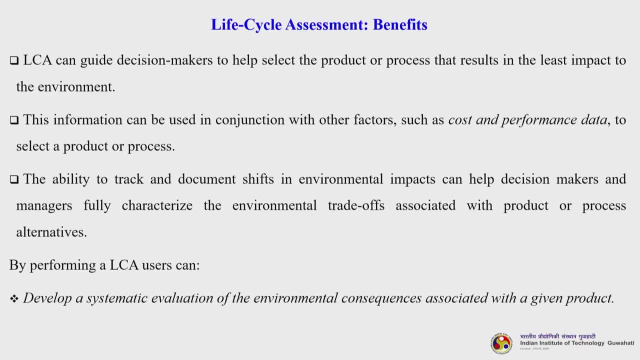 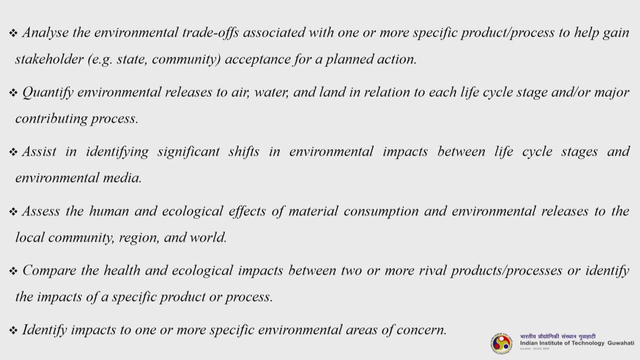 makers and managers fully characterize the environmental trade-offs associated with the product or process alternatives. Now, by performing a LCA, users can what they can do. basically, it is listed out. okay, now develop a systematic evaluation of the environmental consequences associated with a given product. then analyze the environmental trade-offs associated with one or more specific product. 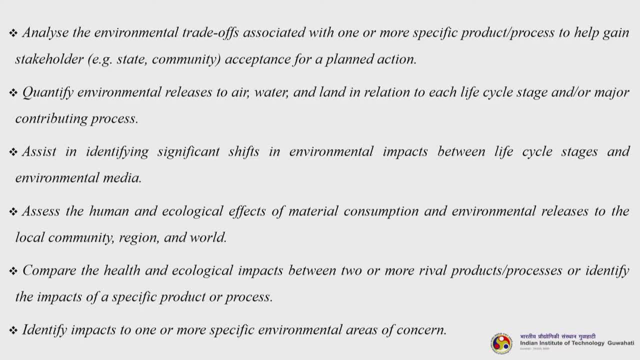 or process to help gain stakeholders, as, for example, state community acceptance for a planned action. Third is quantify environmental releases to air, water and land in relation to each life cycle stage. This is a major, major contributing process. fourth is assist in identifying significant shifts in environmental impacts between life cycle stages and environmental media. then, 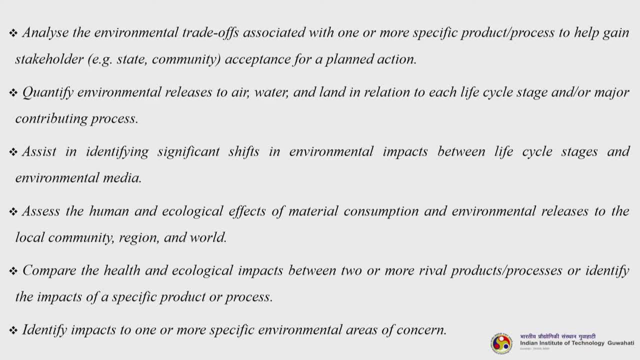 next is assess the human and ecological effects of the material consumption and environmental releases to the local community region as well as the world. next is compare the health and ecological impacts between two or more rival products, processes or identify the impacts of a specific product or processes. and the last one is identify impacts to one or more. 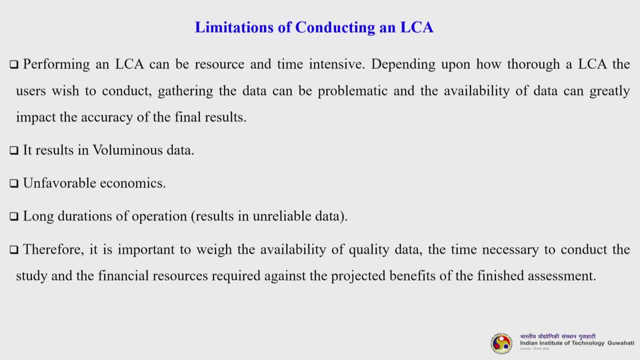 specific environmental areas of concern. Now let us talk about the limitations of conducting an LCA. Now, performing an LCA can be resource or time intensive, depending upon how thorough a LCA the users wish to conduct. gathering the data can be problematic and the availability of 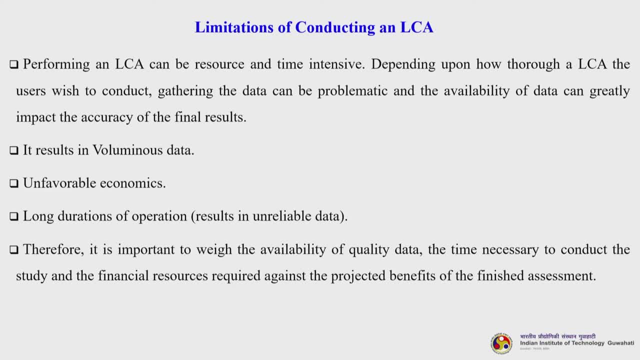 data can greatly impact the accuracy of the final results, So it results in voluminous data. there are unfavorable economical conditions or needs to be taken into consideration Long durations of operation. Basically, that results in unreliable data. therefore, it is important to weigh the availability of quality data, the time necessary to conduct the study and the financial resources required. 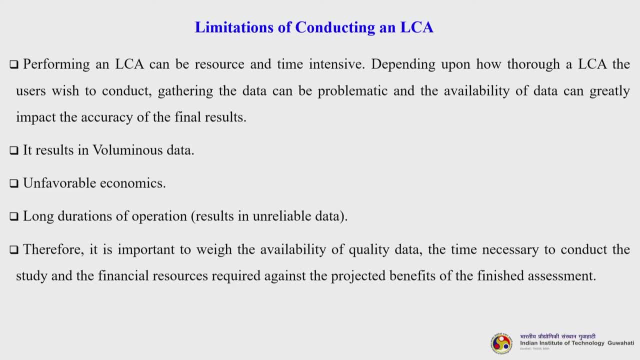 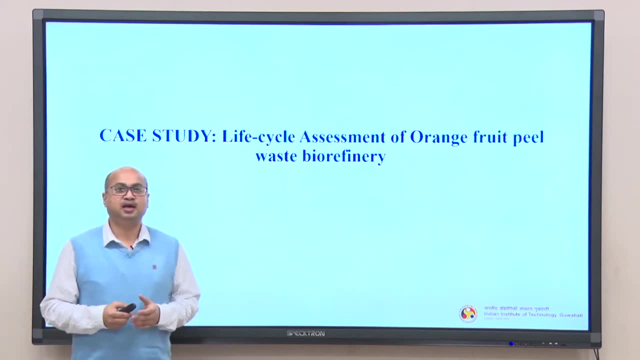 against the projected benefits of the finished assessment. Now let us take a case study. So here I have taken a life cycle assessment of a orange, a fruit peel, waste, biorefinery, correct. you remember we have also taken a case study when we discussed about the techno-economical. 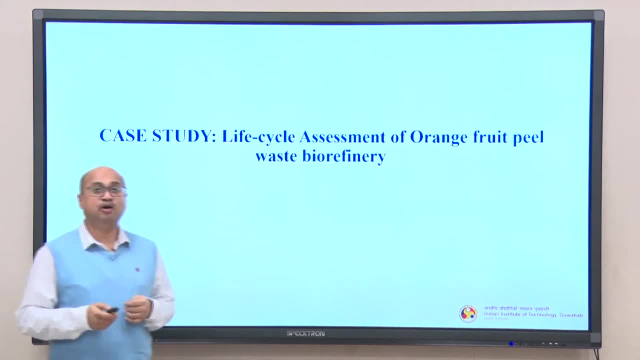 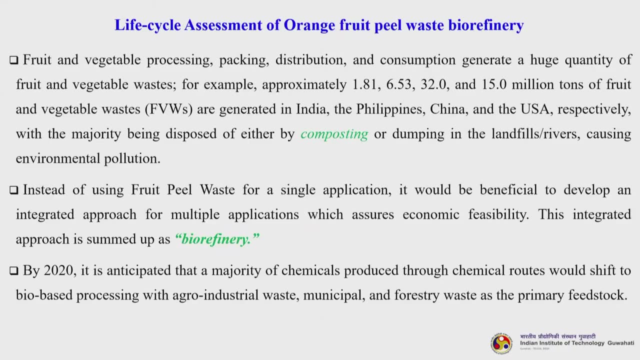 assessment in our last class right. So let us see how LCA has been carried out for this particular waste biorefinery. So fruit and vegetable processing, packing, distribution and consumption generate a huge quantity of fruit and vegetable waste, for example, approximately 1.81,, 6.53,, 32.0 and. 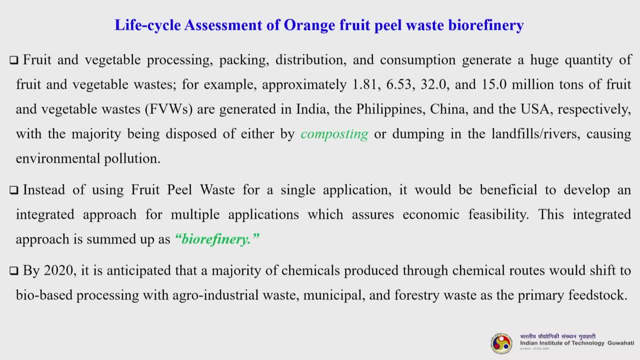 15.0 million tons of fruit and vegetable waste are generated in India, the Philippines, China and the United States respectively. We will discuss about the LCA later, So let us look at another example. Now you can see that the product of a fruit peel waste biorefinery is getting produced. 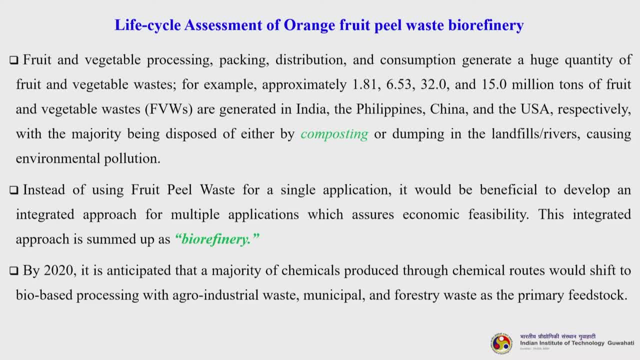 by the biorefinery. So the product of biorefinery is this product of a biorefinery which is being produced by biorefinery. So by 2020 it is anticipated that a majority of chemicals produced through chemical routes 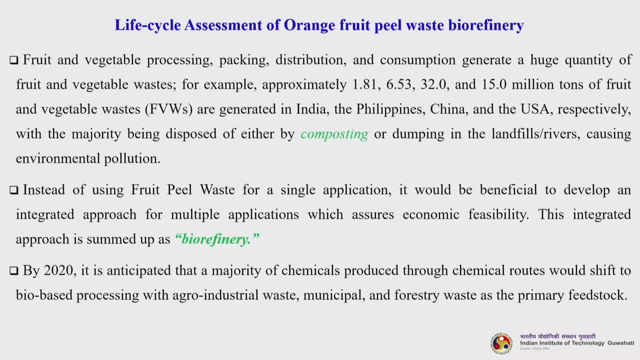 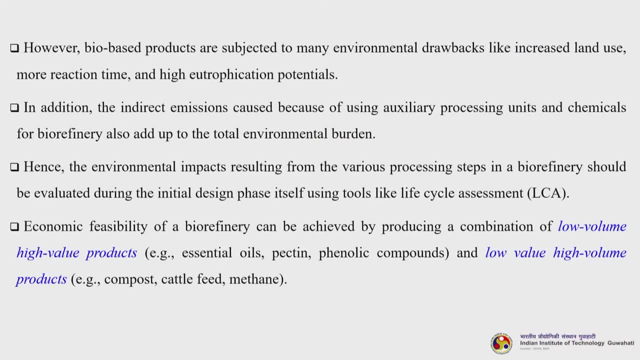 would shift to bio-based processing, with agro-industrial waste, municipal and forestry waste as the primary feedstock. However, bio-based products are subjected to many environmental drawbacks, like increased land use, more reaction time and high eutrophication potentials. In addition, the indirect emissions caused because of using auxiliary processing units. 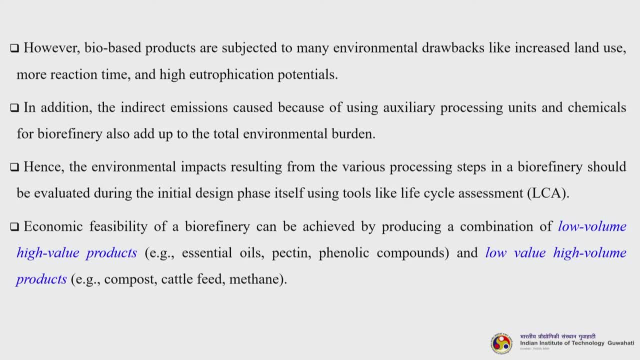 and chemicals for bio-refinery also add up to the total environmental burden. Hence, the environmental impacts resulting from the various processing step in a bio-refinery should be evaluated during the initial design phase itself, using tools like life cycle assessment. Economic feasibility of a bio-refinery can be achieved by producing a combination of: 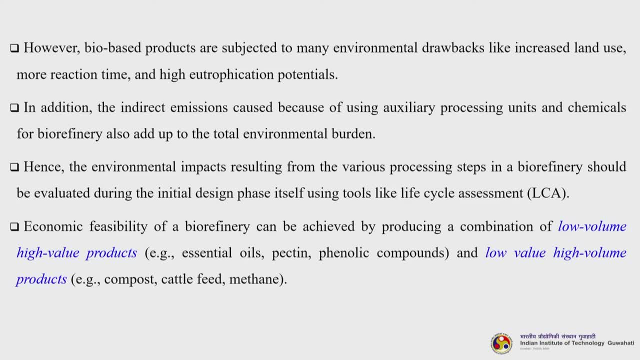 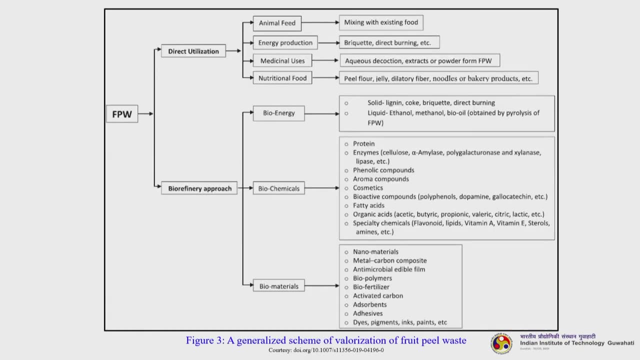 low volume, high value products, as for example essential oils, pectin, phenolic compounds, and also low value, high volume products, For example compost, cattle feed, methane, which are produced in high volume or large volume. So this figure 3 gives us a generalized scheme of the valorization of the fruit peel waste. 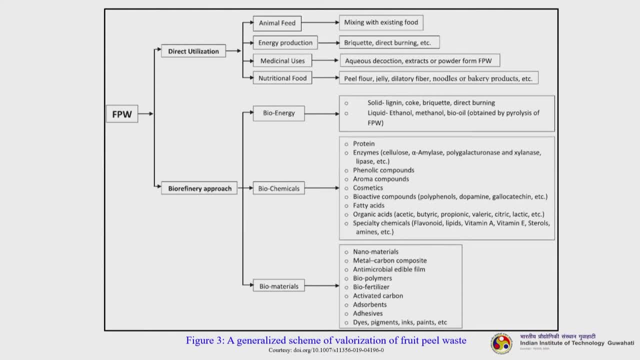 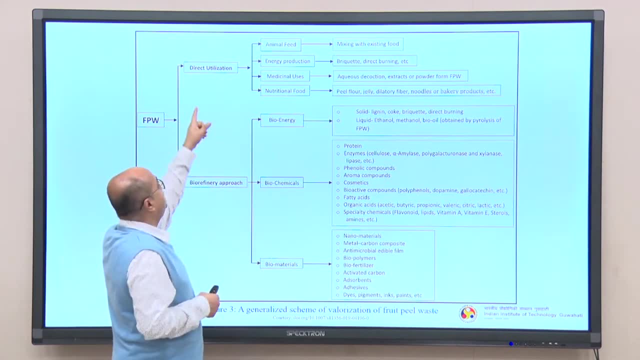 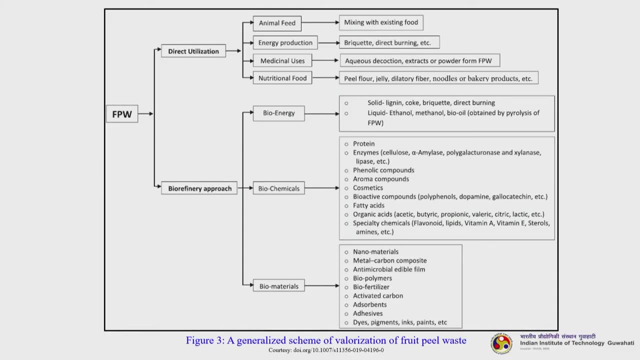 It is a generalized scheme, right, it has been divided into two things. first is a direct approach or direct utilization. second is the bio-refinery approach. Let us see what is the difference. if you go for a direct utilization, you can have animal feed, you can have energy production, you can have some sort of medicinal uses and 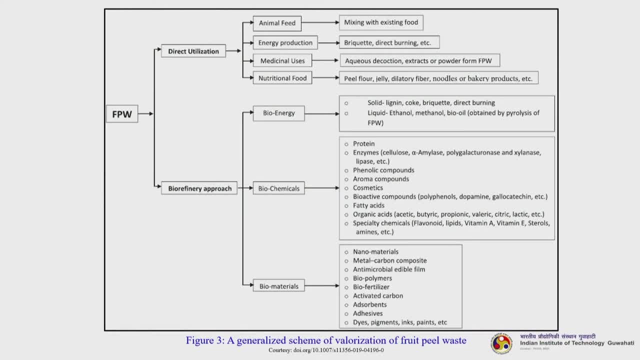 nutritional food components, So mixing with existing food briquette. then there are different things which are noted down. So if you talk about a bio-refinery approach, then we go for various types of multiple products. So it is again divided into three distinct groups. 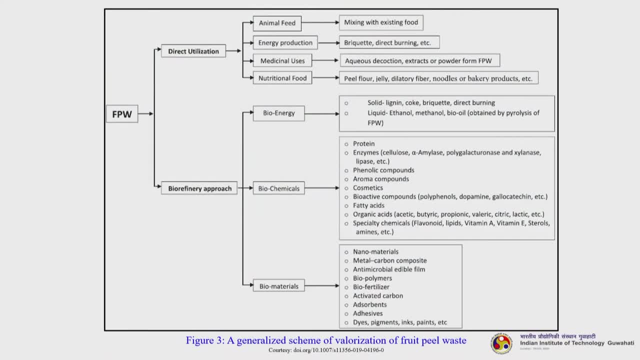 First is bioenergy: biochemicals and then biomaterials. Now in bioenergy we can have solid lignin, coke briquette, direct burning of solid fuel, basically. So you can have liquid ethanol, methanol, as well as bio oil which comes from cycle. 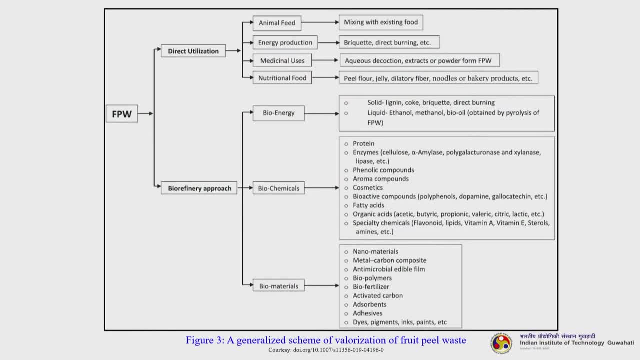 etc. bio oil, which comes from pyrolysis. so this is under bioenergy. Let us see about chemicals now. we can have proteins, enzymes, phenolic compounds, aroma compounds, different types of cosmetics, then bioactive compounds like polyphenols, dopamine. 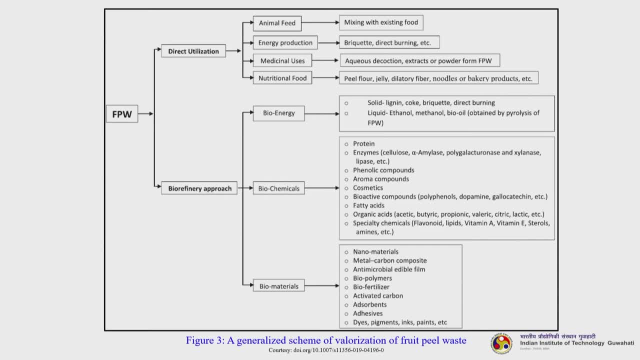 etcetera, fatty acids, organic acids and some specialty chemicals like flavonoids- so many Now. biomaterials: now we can have different types of nanomaterials. we can have metal carbon composite, we can have biopolymers, we can have bio fertilizer, we can have activated 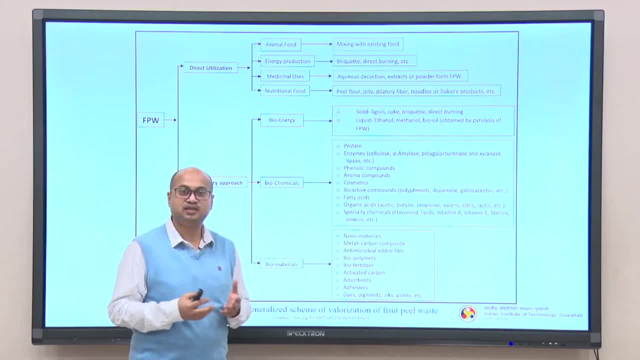 carbon and adsorbents, adhesives, dyes, pigments, inks- so many things You can see now the list is endless- actually in a biorefinery perspective, and we have learned in this particular course that whenever you talk about biorefinery, it should have multiple 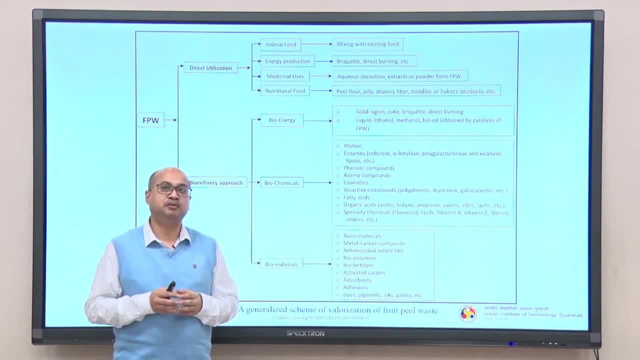 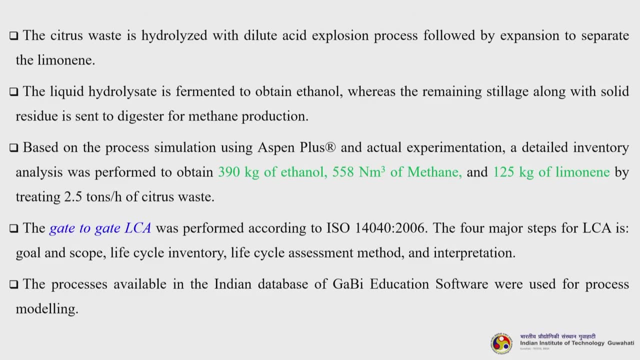 feedstocks. it should have also multiple products. then only it will become sustainable. The citrus waste is hydrolyzed with dilute acid explosion process, followed by expansion to separate the limonene. Now I am just going to discuss that, how this is been carried out. 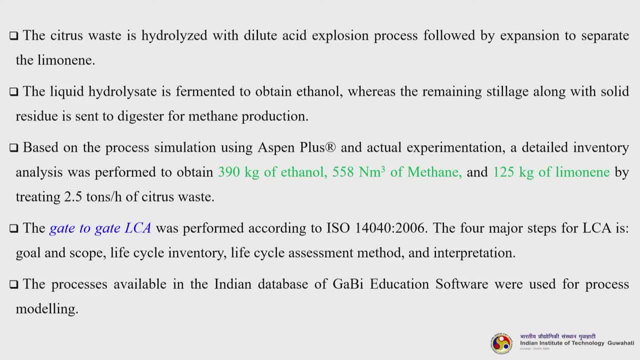 That means how the biorefinery actually study has been done and what are the assumptions has been taken. all these things we are going to discuss. okay, So the liquid hydrolyzed is fermented to obtain ethanol, whereas the remaining stillage along. 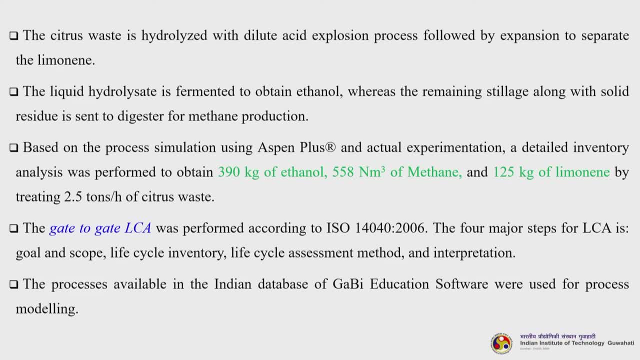 with the solid residue is sent to digester for methane production, basically anaerobic digestion. Now based on the process simulation using Aspen plus and actual experimentation, a detailed inventory analysis was performed to obtain 390 kg of ethanol, 558 Nm cube per liter of. 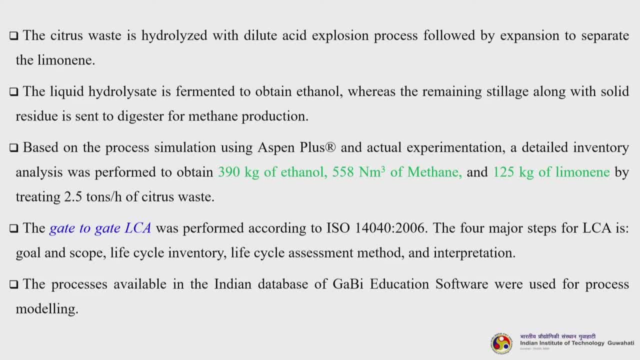 methane and 125 kg of limonene by treating 2.5 tons per hour of citrus waste. Now the gate to gate. LCA was performed according to the ISO 140402006.. The four major steps for LCA is goal and scope, life cycle inventory, life cycle assessment. 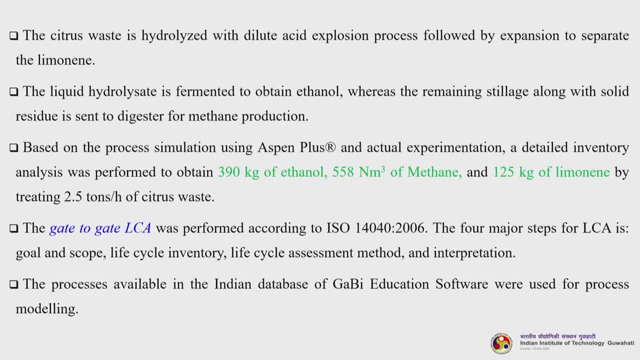 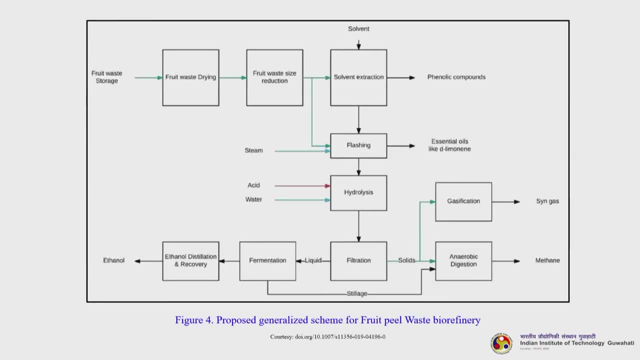 as interpretation. This we have already discussed. okay, Now the processes available in the Indian database of the Gavi education software were used for the process modeling. This is the proposed generalized scheme for the fruit peel waste biorefinery. Now you can see that the fruit waste storage, it goes to drying. then size reduction: mechanical. 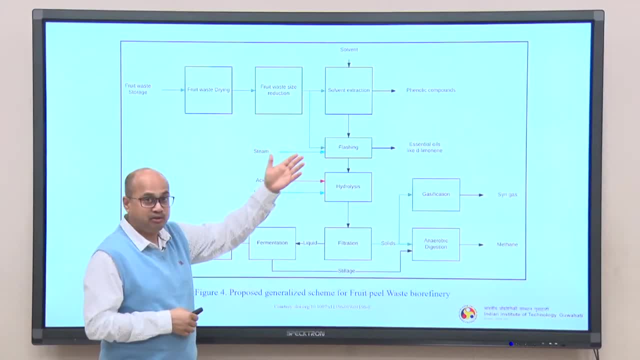 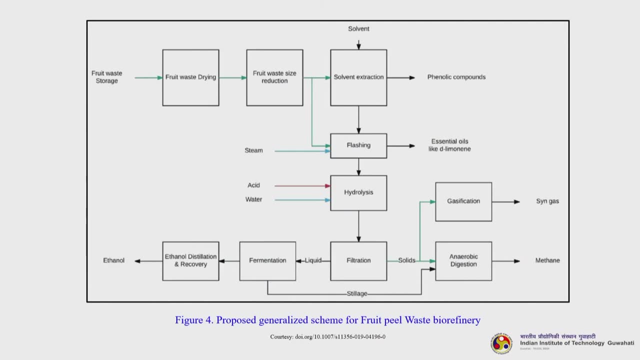 operation basically okay. Then you go for solvent extraction where you take out the phenolic compounds, then whatever left out, that goes to flushing. so again you get essential oils as a byproduct from that side. okay, You steam here. then it goes for the hydrolysis part. okay. 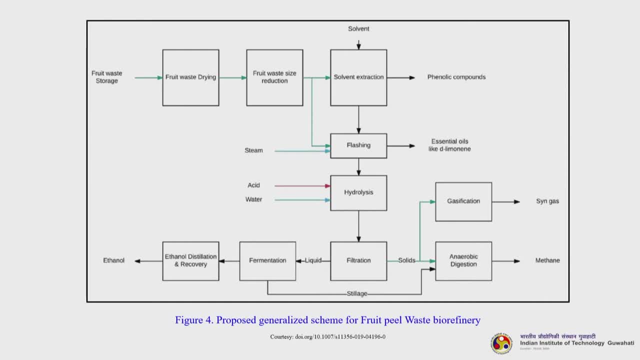 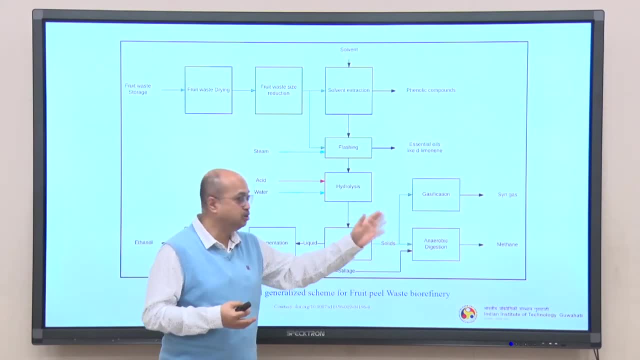 Here you use acid and water and then you filter it. once you filter, there is a liquid part, there is a solid part. Solid part goes to anaerobic digestion. you get methane. part of that can also can be gasified to produce seed gas. 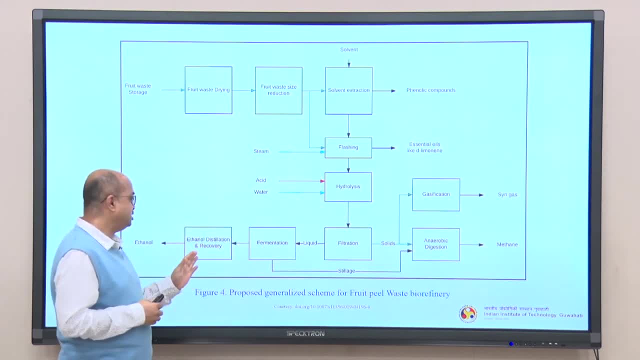 Now the liquid product, okay, can be fermented. then you get ethanol, distillation and recovery. basically, you are producing ethanol distillate, finally ethanol- okay. Then part of the fermentation, if the broth, the stills, can be fed to anaerobic digestion. 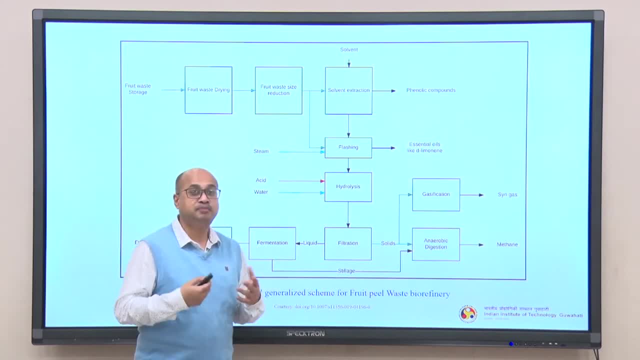 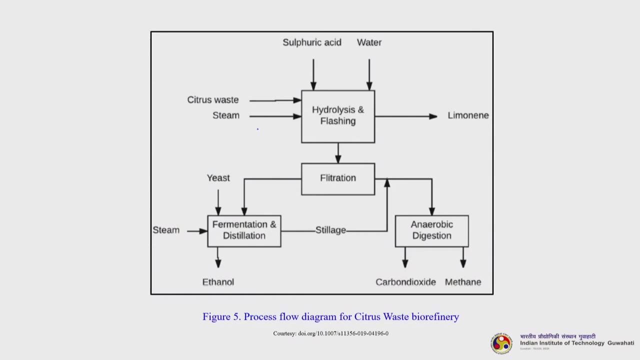 okay, It has so many valuable components which can be used as nutrients. source of nutrients, nutrient during anaerobic digestion. So this is a simply popular way. Okay, simplified schematic representation of the fruit field waste biorefinery. Now this process flow diagram tells us about the citrus waste biorefinery. here you can. 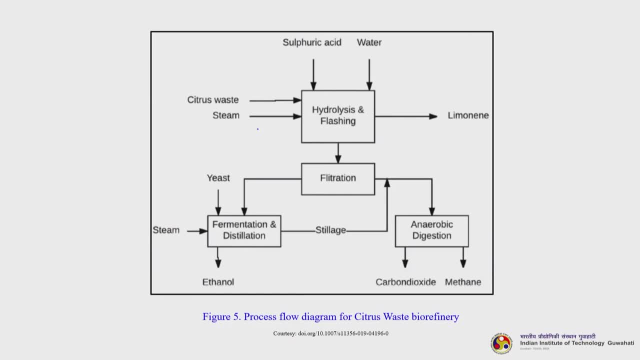 see that hydrolysis and flushing- it is just been expanded little from that side. Citrus, waste steam seed and water dilute sulfuric acid treatment. you carry out hydrolysis and flushing. you get limonene, one of the major component of this particular waste biorefinery. 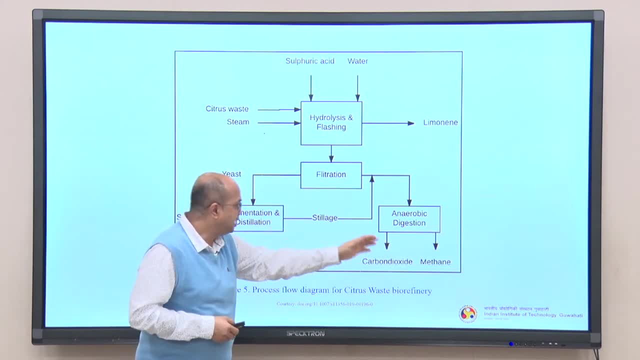 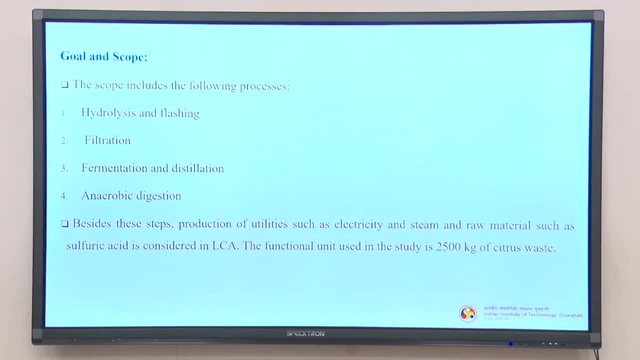 Then, whatever the left out has been filtered, the solid goes to anaerobic digestion, the liquid goes to fermentation: distillation- ethanol using the yeast saccharomyces cerevisiae. Now let us talk about the goal and scope for this particular waste: biorefinery. 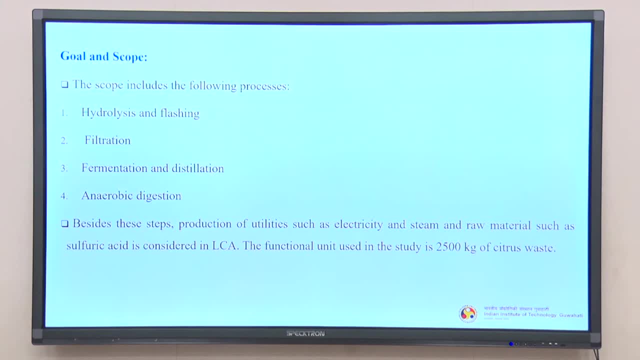 Now the scope includes the following processes: hydrolysis and flushing, filtration, fermentation and distillation, then anaerobic digestion- the four major processes. Now, besides these steps, production of utilities such as electricity and steam and raw materials such as sulfuric acid is considered in the LCA. 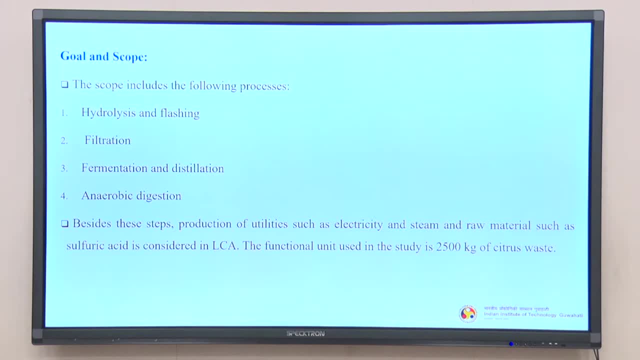 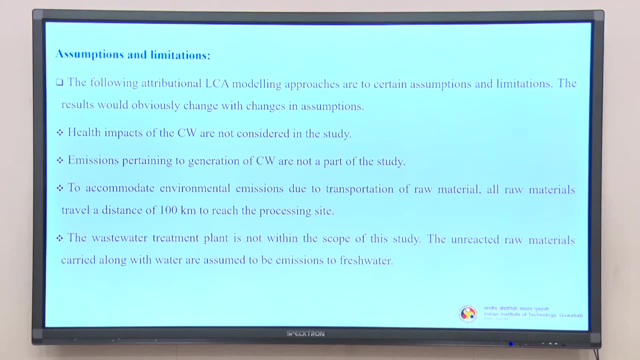 The functional unit used in the study is 2000.. 500 kg of citrus waste. Now assumptions and limitations. now the following attributional LCA modeling approaches are to certain assumptions and limitations. the results would obviously change with the change in assumptions. First is that health impacts of the CW are not considered in this, in this study. ok, 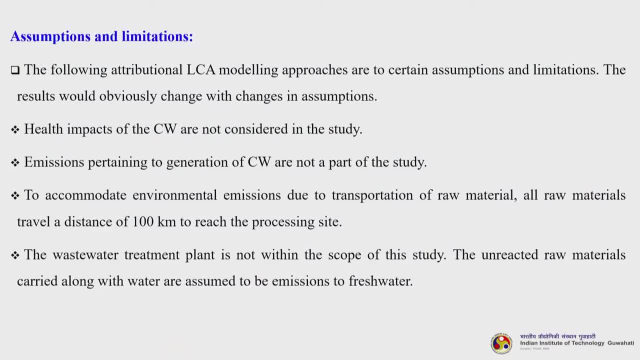 Second, emissions pertaining to the generation of CW are not a part of this study. Third, to accommodate environmental emissions due to transportation of the raw materials, all raw materials travel a distance Distance of only 100 kilometer to reach the processing site. Fourth, the wastewater treatment plant is not within the scope of the study. the ETP ok effluent. 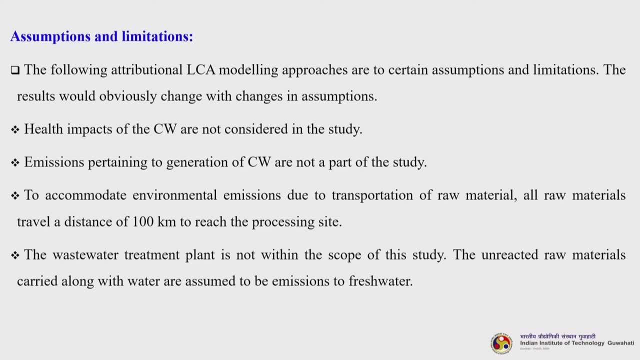 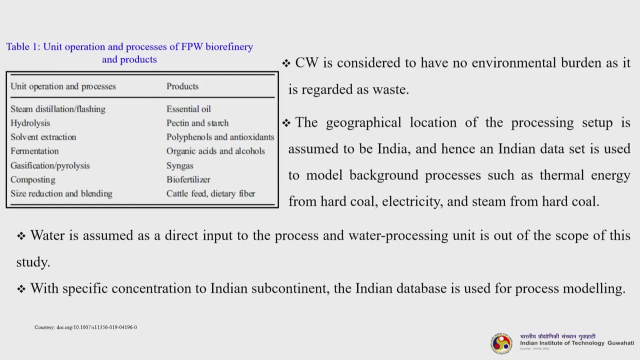 treatment plant. The unreacted raw materials carried along with water are assumed to be emissions to fresh water. So the table lists the different types of unit operations and processes of the PW biorefinery and products. If you talk about steam distillation, flushing the product is essential oil hydrolysis, the 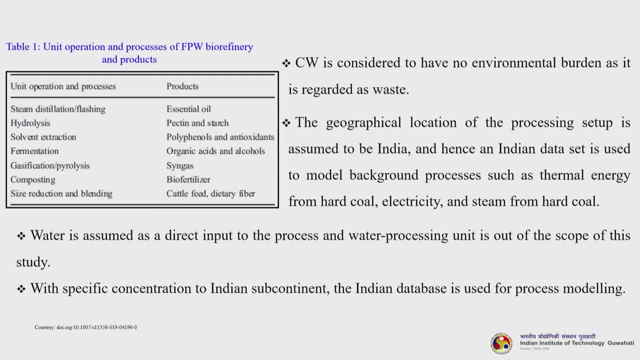 product is pectin and starch. We get polyphenols and antioxidants. Fermentation, we get organic acids and alcohols like ethanol, ok, Gasification and pyrolysis. we get syngas, Composting, we get biofuel, laser size reduction and blending. we get cattle feed and dietary. 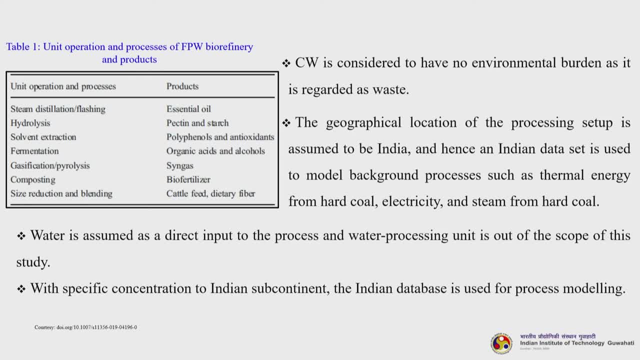 fiber. Now CW is considered to have no environmental burden as it is regarded as waste. The geographical location of the processing set up is assumed to be India, and hence an Indian dataset is used to monitor the quality of the products, to model background processes such as thermal energy from hard coal, electricity and steam. 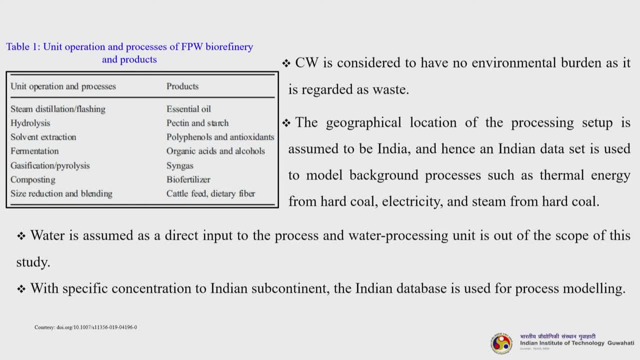 from hard coal. water is assumed as a direct input to the process, and water processing unit is out of the scope of this study, With specific concentration to Indian subcontinent. the Indian database is used for process modeling. Then let us talk about the life cycle inventory. the first one is feedstock. 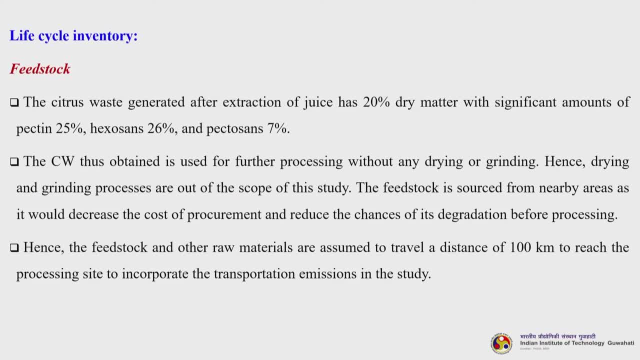 Now the citrus waste generated after extraction of juice has 20% dry matter with significant amounts of pectin, that is, 25%, hexazones almost 26% and pectozones 7%. The CW thus obtained is used for further processing without any drying or grinding. 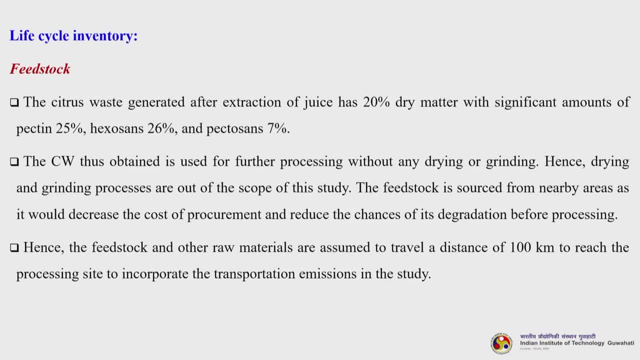 Hence drying and grinding processes are out of the scope of this particular study. The feedstock is sourced from nearby area, as it would decrease the cost of procurement and reduce the chances of its degradation before processing. Hence the feedstock and other raw materials are assumed to travel a distance of 100 kilometer. 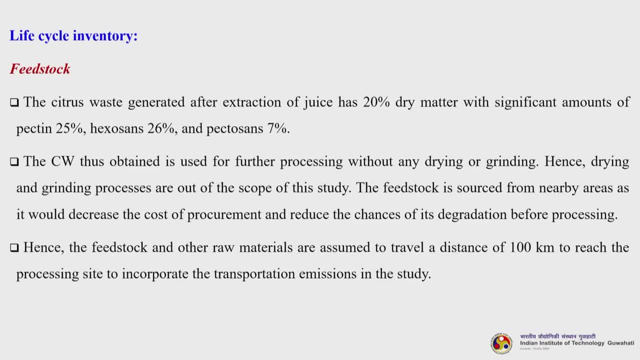 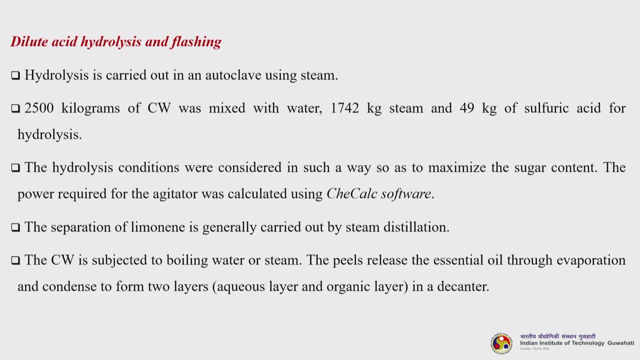 to reduce the chances of its degradation before processing. To reach the processing site, to incorporate transportation emissions in the study, Then the next method is dilute acid hydrolysis and flushing. Now hydrolysis is carried out in an autoclave using steam. 2500 kilogram of CW was mixed. 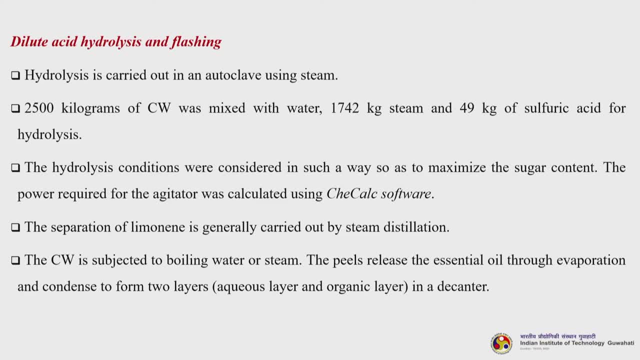 with water, 1742 kilogram of steam and 49 kilogram of sulfuric acid. for hydrolysis, The hydrolysis conditions were considered in such a way so as to maximize the sugar content. The power required for the agitator was calculated using. 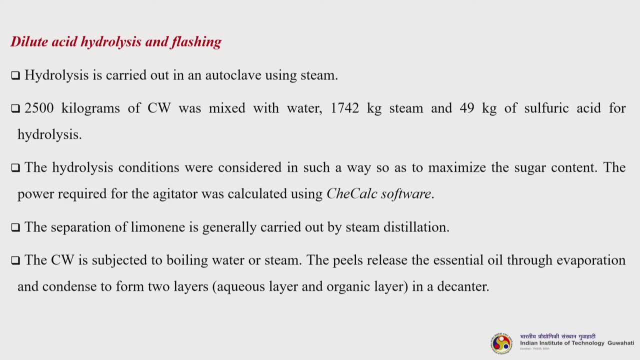 the C-H-E-C-L-C software. the separation of limonene is generally carried out by steam distillation. The CW is subjected to boiling water or steam. The pills release the essential oil through evaporation and condense to form two layers. 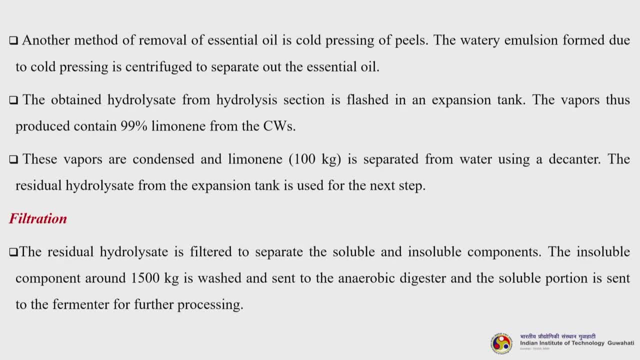 a coarse layer and organic layer in a decanter. Another method of removal of essential oil is cold pressing of pills. The watery emulsion formed due to cold pressing is centrifuged to separate out the essential oil. The obtained hydrolysate from hydrolysis section is flushed in an expansion tank. 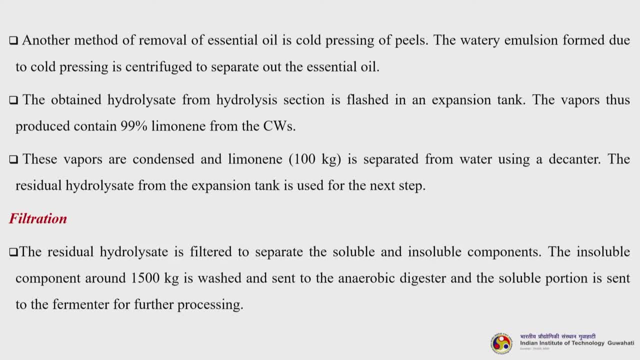 The vapors thus produced contain 99 percent limonene from the CWs. Now these vapors are condensed and limonene that is 100 kg is separated from water using a decanter. The residual hydrolysate from the expansion tank is used for the next step, filtration. 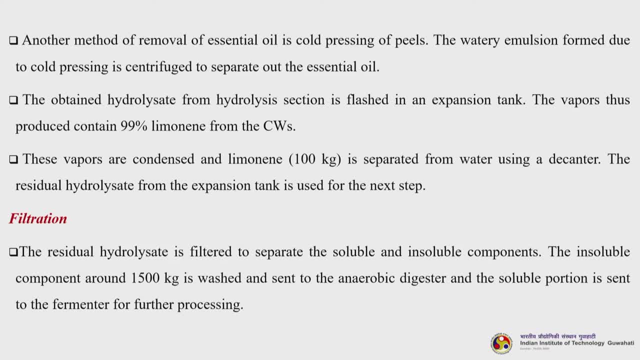 The residual hydrolysate is filtered to separate the soluble and insoluble components. the insoluble component- around 1500 kg, 500 kilogram- is washed and sent to the anaerobic digester and the soluble portion is sent to fermenter for further processing for anaerobic digestion to carried out. actually, okay. 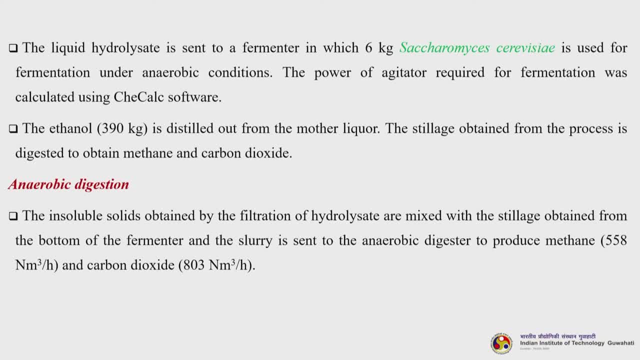 Now the liquid hydrolysis is sent to a fermenter in which 6 kilograms of Saccharomyces cerevisiae is used for fermentation under anaerobic conditions. The power of agitator required for fermentation was calculated using the CHECLC software K-Calc. 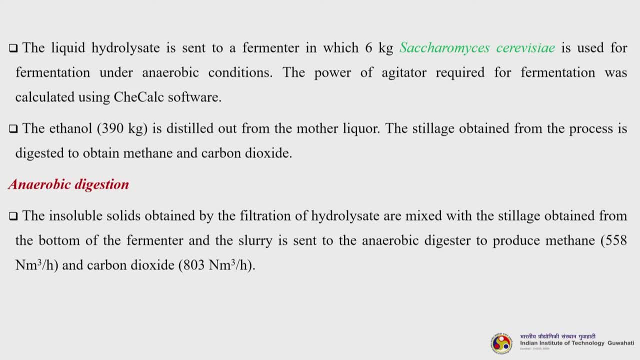 software. okay. the ethanol, that is 390 kg, is distilled out from the mother liquor. the stillage obtained from the process is digested to obtain methane and carbon dioxide. Then the next one is the anaerobic digestion: the insoluble solids obtained by the filtration. 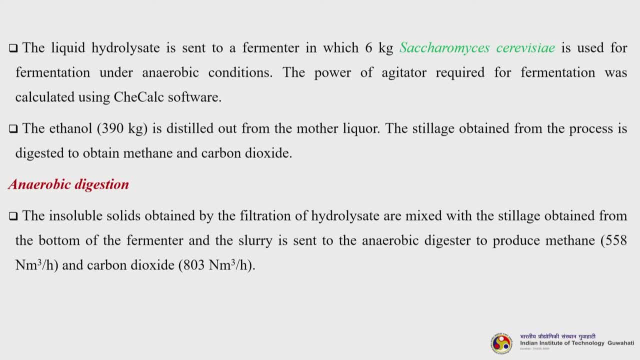 of hydrolysis are mixed with the stillage obtained from the bottom of the fermenter and the slurry is sent to the anaerobic digester to produce methane 558 nmq per hour and carbon dioxide is almost 803 nmq per hour. 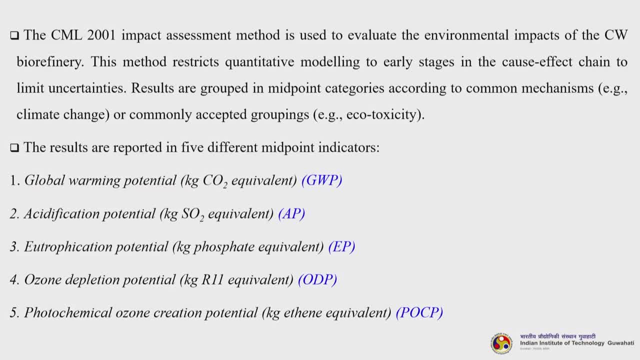 Now the CML200 2001 impact assessment method is used to evaluate the environmental impacts of the CW biorefinery. This method restricts quantitative modeling to early stages in the cause effect chain. to limit uncertainties, Results are grouped in midpoint categories according to common mechanism, such for example: 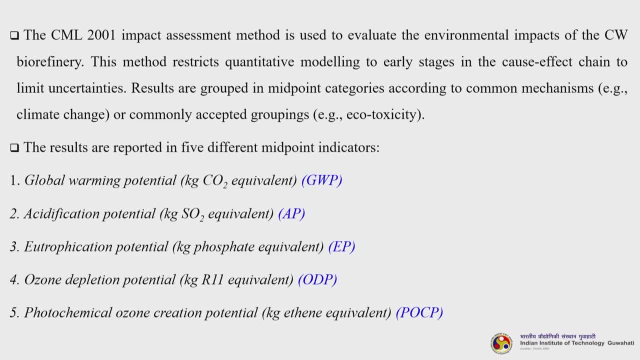 climate change or commonly accepted grouping such, for example, ecotoxicity. The results are reported in 5 different midpoint indicators. First is global warming potential. that is measured in kilograms of carbon dioxide equivalent. Second is acidification potential. it is measured in kilogram per sulphur dioxide equivalent. 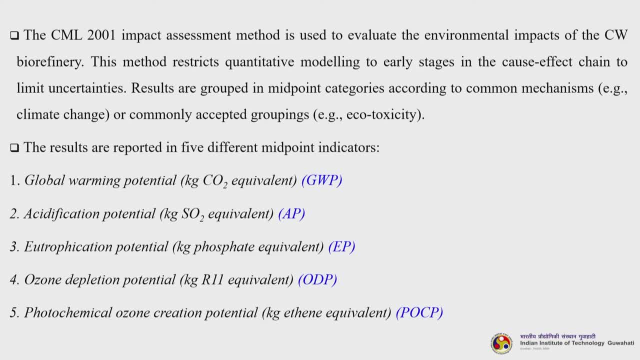 Third is eutrophication potential. it is measured in kilogram of phosphate equivalent. Fourth is ozone depletion potential. it is measured in kilogram of R11 equivalent. and the final one is photochemical ozone creation potential. it is again measured in terms of kilograms per ethane equivalent. okay, 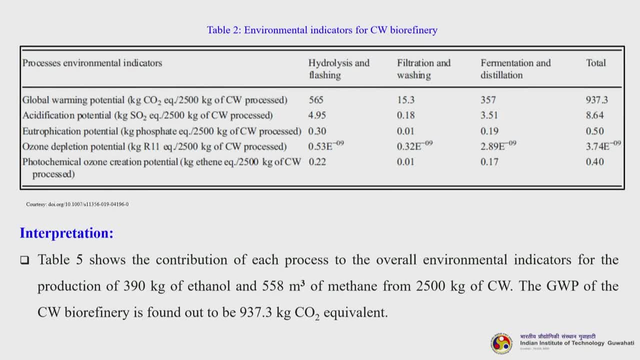 So these five major parameters are very important, Thank you. So this table will give you an understanding about the environmental indicators for this particular CW biorefinery. okay, You can see that. global warming potential: okay. So kilogram carbon dioxide equivalent per 2500 kilograms of CW that is processed. 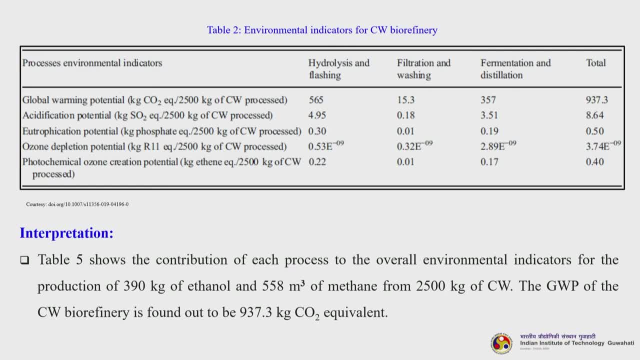 So, from the hydrolysis and flushing, it is 565. filtration and washing step, it is 15.3. fermentation and distillation is 357. total is 937.3. okay, That is 937.3.. So this is 937.3 kilograms of carbon dioxide equivalent per 2500 kilogram of CW. that is. 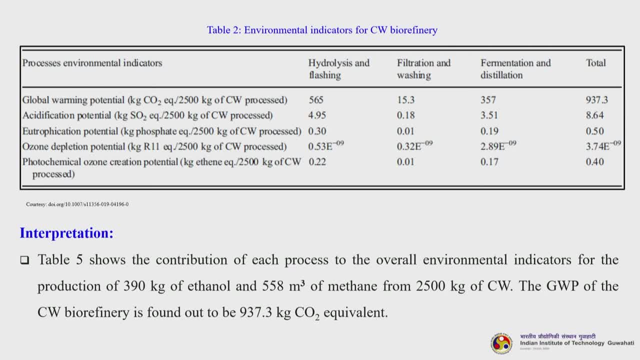 processed. Now let us talk about this eutrophication potential. okay, So it is 0.5, very small okay for again 2500 kilogram of CW process. if you talk about that photochemical ozone creation potential, it is 0.4 kilogram ethane equivalent for 2500 kilogram. 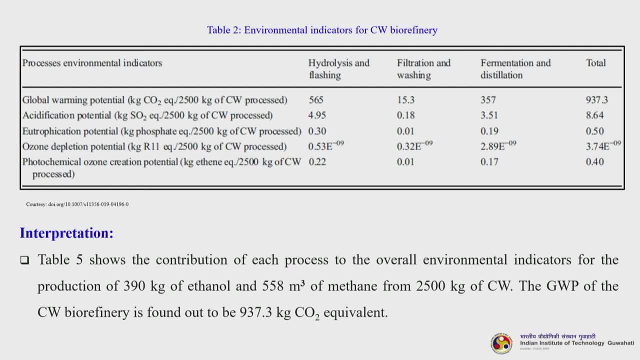 per the of the CW that is processed. Fine, So this gives you an understanding about how different types of these processes are generating different types of parameters, which we have measured in exclusively five different indicators. right, The next is interpretation. Now the table five. I think there is a mistake here. it will be table two. 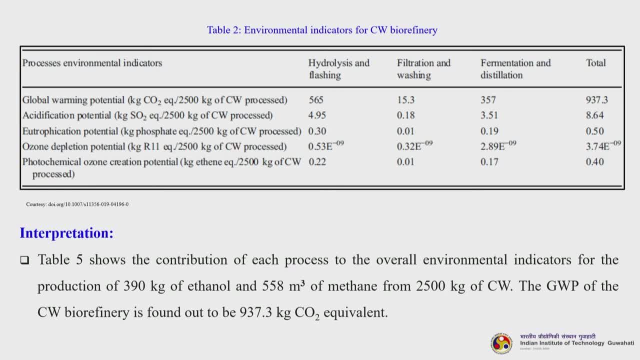 Table two shows the contribution of each process to the overall environmental indicators for the production of 390 kg of ethanol and 558 meter cube of methane from 2500 kg of CW. Okay, Thank you. So the GWP of the CW biorefinery is found out to be 937.3 kg carbon dioxide equivalent. 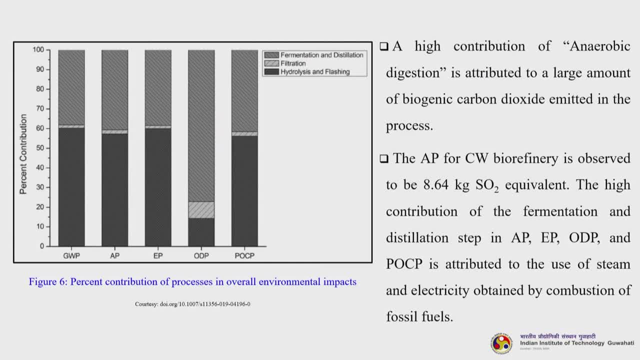 So if you look into this particular figure six, it tells us about the percent contribution of processes in overall environmental impacts. okay, Again for this, five different indicators. a high contribution of anaerobic digestion is attributed to a large amount of biogenic carbon dioxide emitted in the process. you can see. 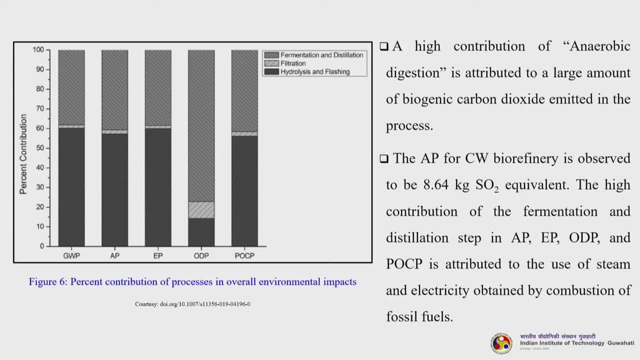 that during anaerobic digestion It is Correct Then. the AP for CW biorefinery is observed to be 8.6 per kilogram sulphur dioxide equivalent. The high contribution of the fermentation and distillation steps in AP, EP, ODP and POCP. 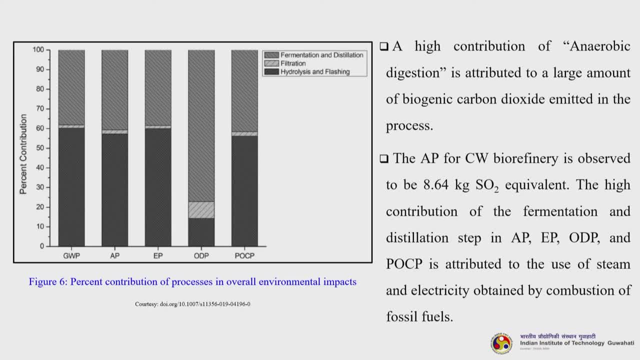 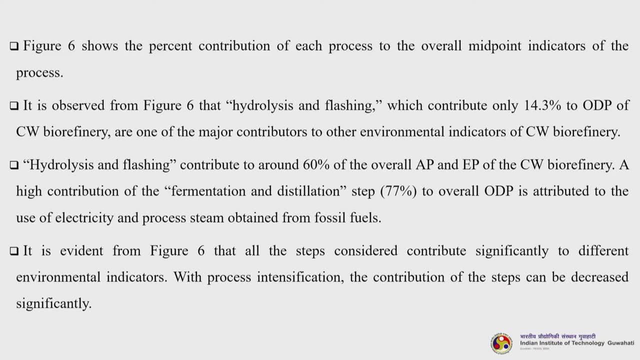 is attributed to the use of steam and electricity obtained by combustion of fossil fuels. So figure six shows the percent contribution of each process to the overall midpoint indicators of the process. It is observed from this figure that hydrolysis and flushing- That contributes only 14.3 percent of ODP of the entire CW biorefinery- is one of the major 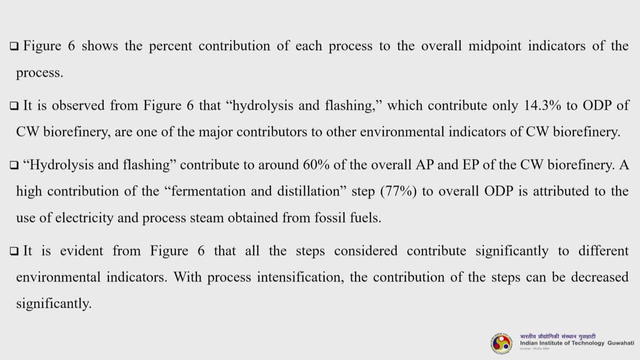 contributors to other environmental indicators of this particular biorefinery. Hydrolysis and flushing contribute to around 60 percent of the overall AP and EP of the CW biorefinery. A high contribution of the fermentation and distillation step, almost 77 percent to overall. 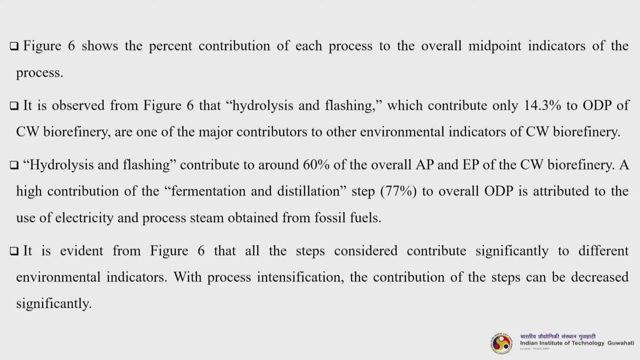 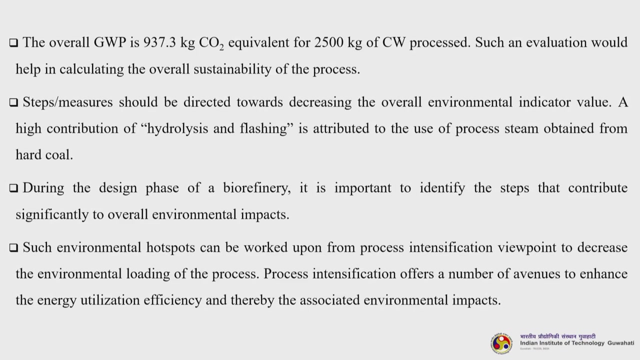 ODP is attributed to the use of electricity and process steam obtained from fossil fuels. It is evident from figure six That all the steps considered contribute significantly to different environmental indicators. with process intensification, the contribution of the steps can be decreased significantly. The overall GWP is 937.3 kilogram of carbon dioxide, equivalent for 2500 kilogram of CW. 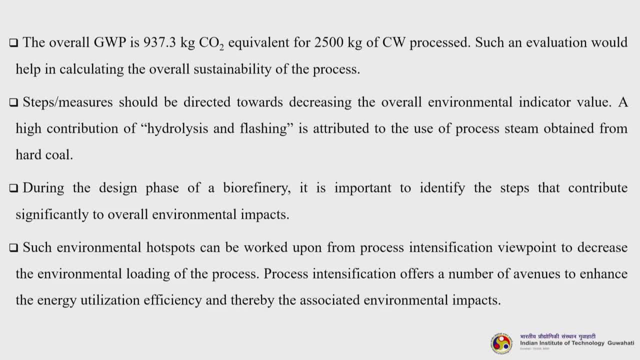 process. such an evaluation would help in calculating the overall sustainability of the process. Steps and measures should be directed towards decreasing the overall environmental indicator value. A high contribution of hydrolysis and flushing is attributed to the use of process steam obtained from the hard coal. 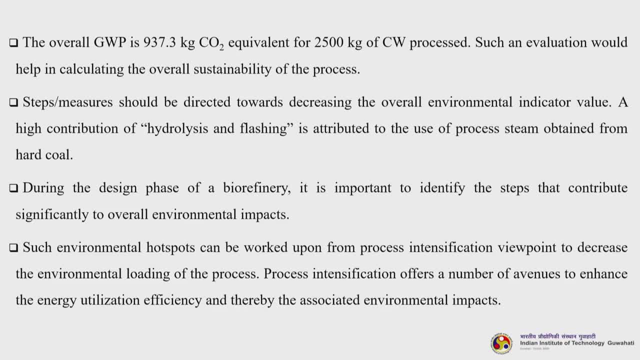 During the design phase of a biorefinery, it is important to identify the steps that contribute significantly to overall environmental impacts. Such environmental hotspots can be worked upon from process intensification viewpoint to decrease the environmental loading of the process. Process intensification offers a number of avenues to enhance the energy utilization. 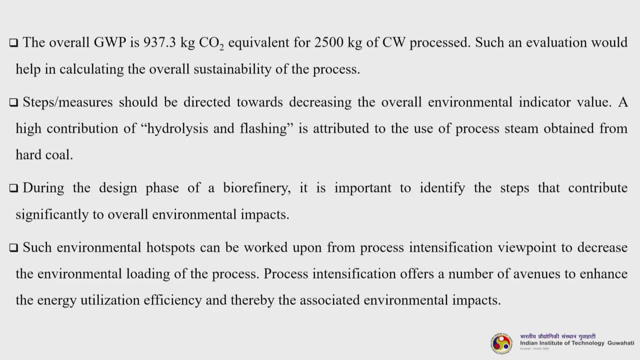 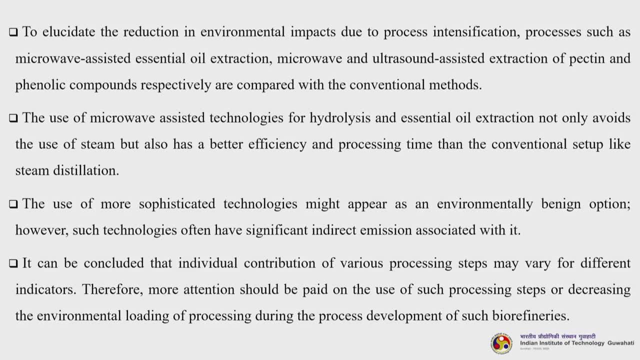 efficiency. The environment impacts are immediate and associated their environmental impacts. So, to elucidate the reduction in environmental impacts due to process intensification, processes such as microwave assisted essential oil extraction, microwave and ultrasound assisted extraction of pectin and phenolic compounds respectively, are compared with the conventional methods. 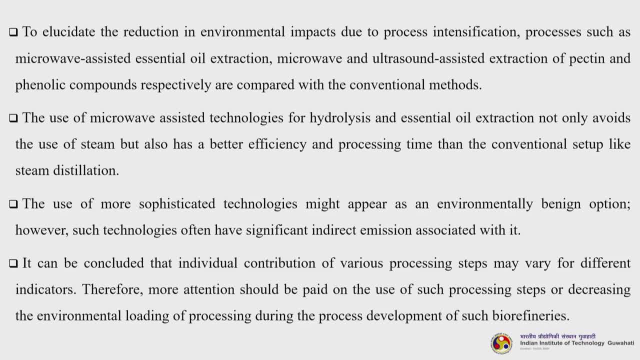 The use of microwave assisted technologies for hydrolysis and essential oil extraction, not only avoiding the use of steam but also has a better efficiency and processing time, then the conventional methods setup, like steam distillation. The use of more sophisticated technologies might appear. 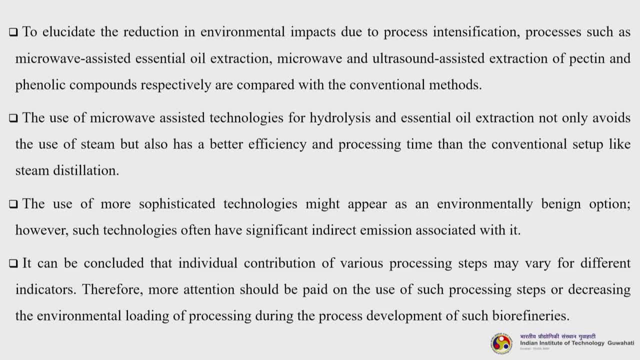 as an environmentally benign option. However, such technologies often have significant indirect emission associated with it. It can be concluded that individual contribution of various processing steps may vary for different indicators. Therefore, more attention should be paid on the use of such processing steps or decreasing the environmental loading of processing during the process development. 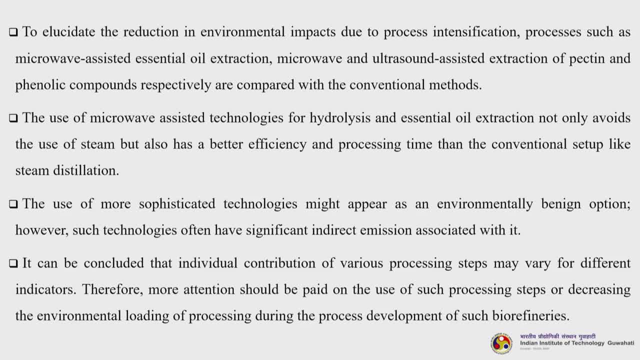 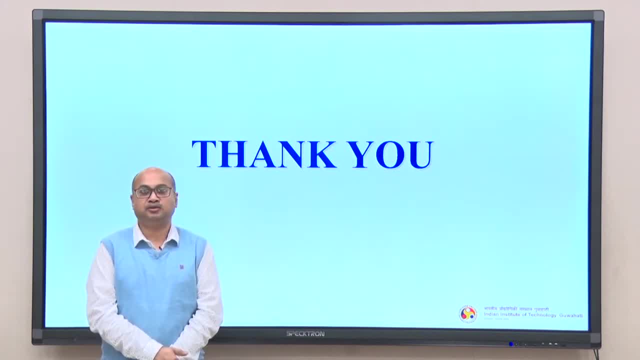 of such biorefineries. So I hope that you got an exclusive idea about what is LCA, how LCA can be carried out Now. so with this I conclude this today's lecture, as well as the entire course. I am hopeful that you have understood the concepts of how biomass can be converted using various 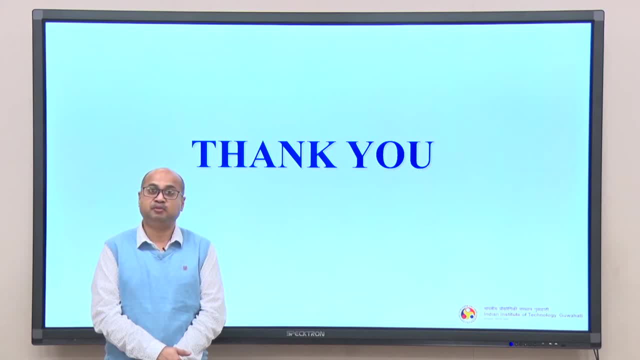 techniques. Then, what is a biorefinery? what are the different types of biorefinery that existed or are being planted? grant in with a reference to the sustainable development goals then also, we have discussed so many different success stories for different conversion technologies. we have also discussed: 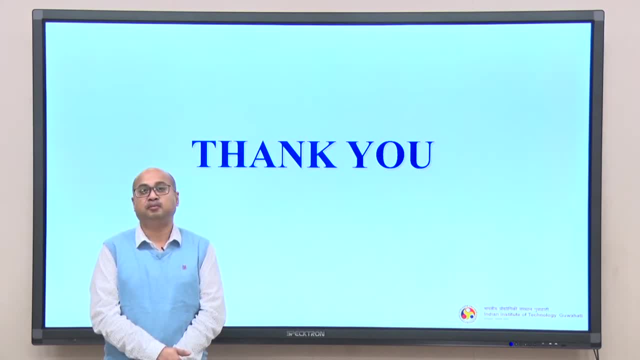 different success studies which are commercially actually running by refineries. then in the fact end of the lecture, we have discussed about the techno-economical assessment and evaluation as well as the life cycle assessment and evaluation. so I am hopeful that this course will be very, very useful for your academic and research purposes, or even somebody wishes. 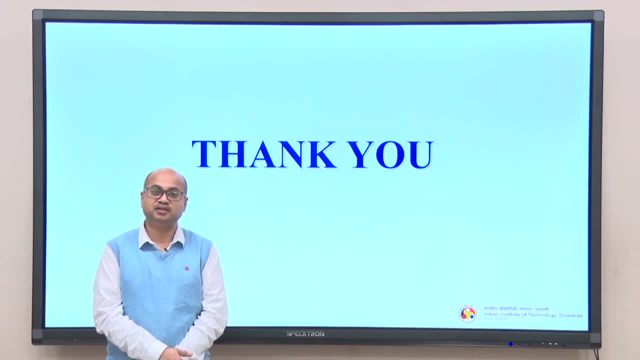 to set up industries, that is, basically biomass batch industries. also. this course will be very helpful for them. so thank you very much. if you have any query, you can feel free to write to me at kmohanty at iitgacin or register your this one query in the SWAMM portal itself.